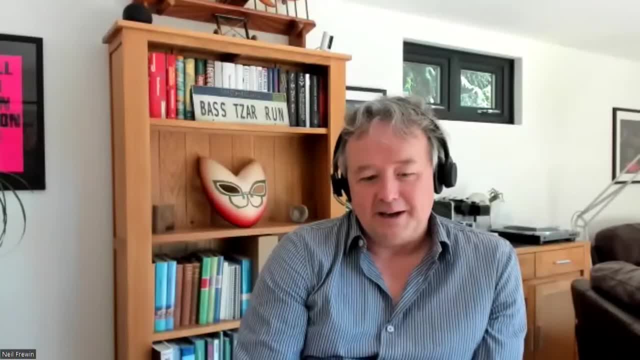 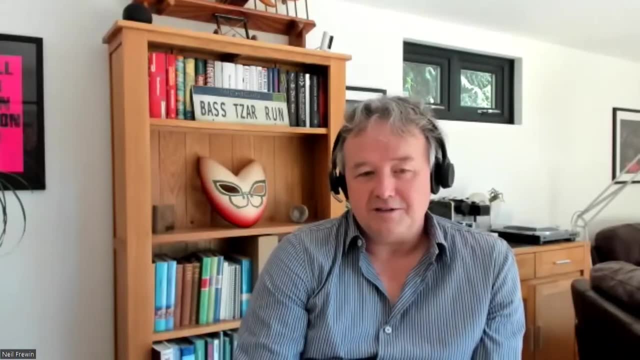 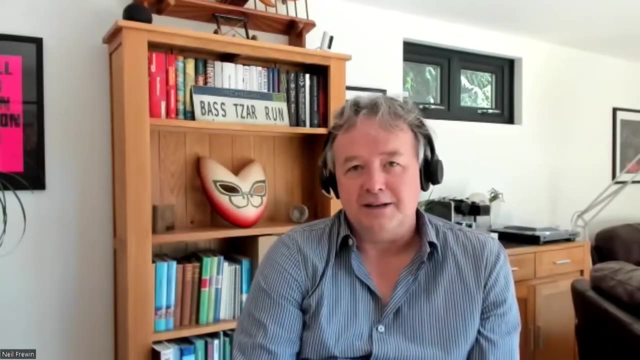 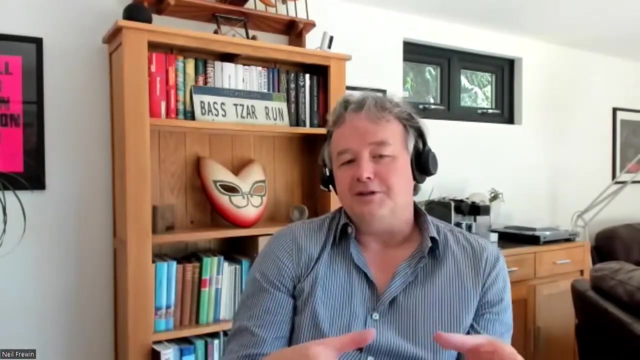 various aspects of geoscience. I'm currently working and leading a team of specialist geoscientists in London, So that includes different topics, areas such as biostratigraphy, structural geology, base modeling, geochemistry- So a lot of the tools that geologists would use within the oil and gas industry. but perhaps 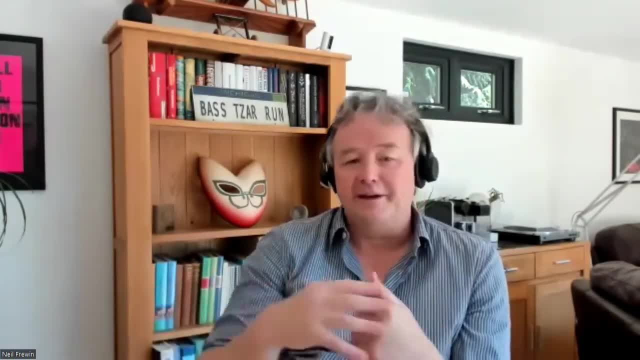 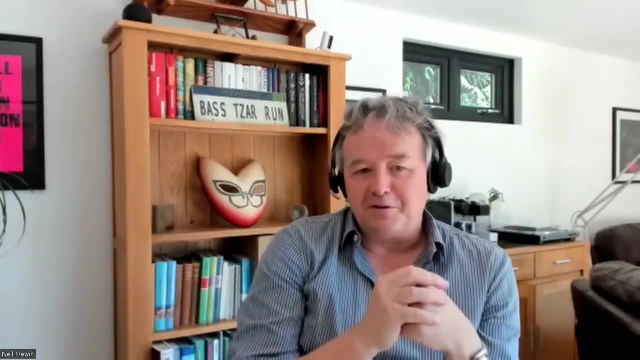 are a bit more expert and niche and specialized than most companies would deploy across the whole organization. So we look after some of those very specialist skills now, which is great. actually, It's really enjoyable. I do a lot of other stuff outside of geoscience. 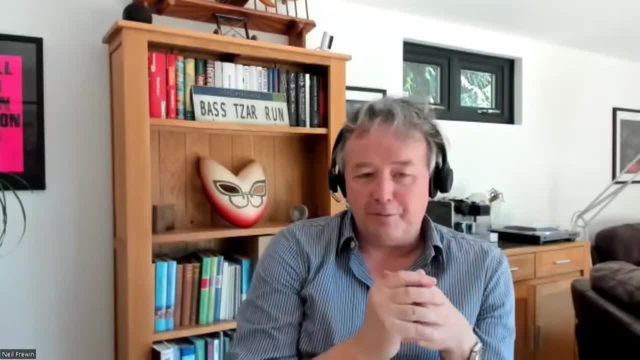 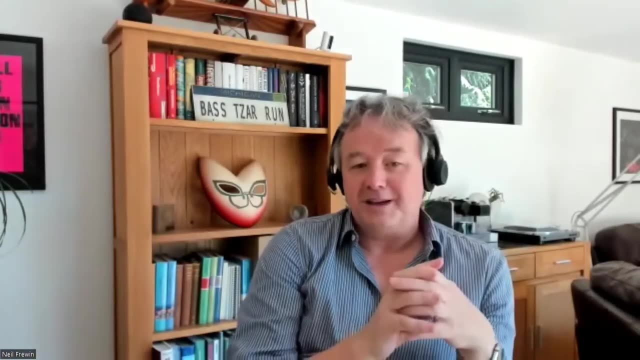 I do a lot of other stuff outside of Shell. I'm a trustee and on the board of the Geological Society of London, And I was president of the Petroleum Exploration Society of Great Britain as well a few years ago. I'm still very active with them. We create conferences. 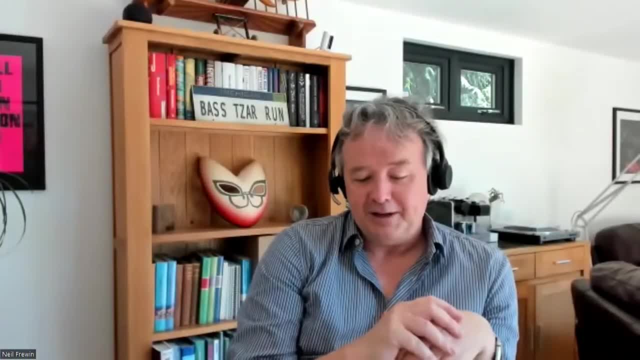 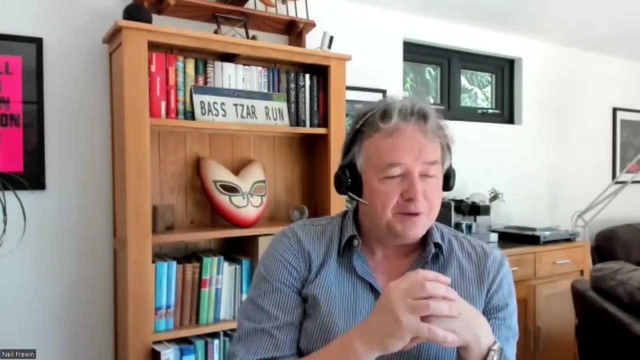 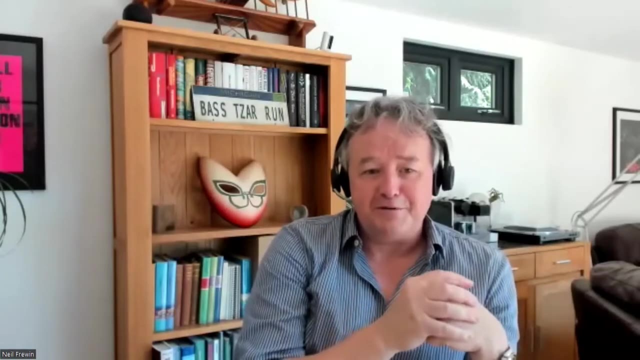 and events around our profession. And then, finally, I'm also a trustee of the Etches Collection, which is a beautiful museum on the south coast of England, where there's a guy who was a plumber- actually, He was fixing taps and pipes for most of his life. 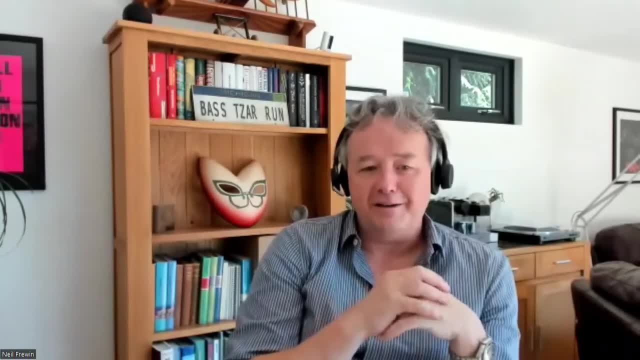 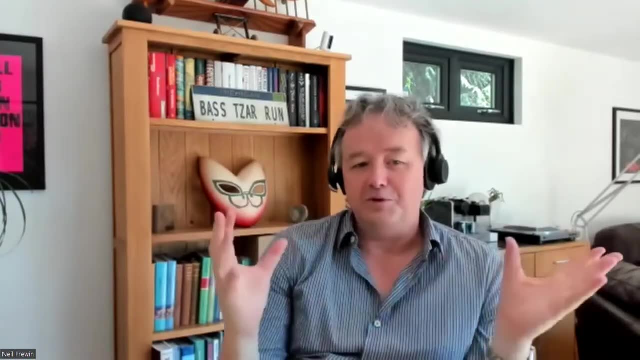 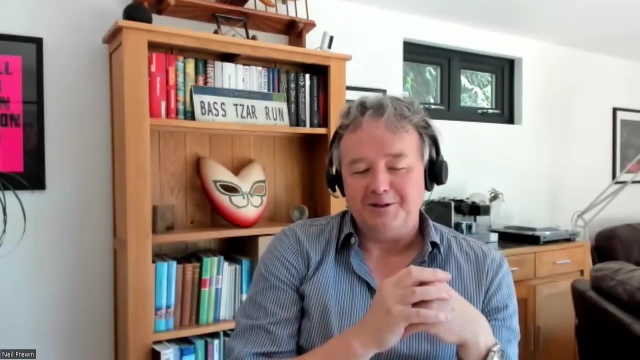 But also he was collecting some of the most astounding fossils you'll ever find in the Kimmeridgian section of the Jurassic, And so he's created a whole museum around these amazing fossils And you can go there and see a complete ecosystem, which is really 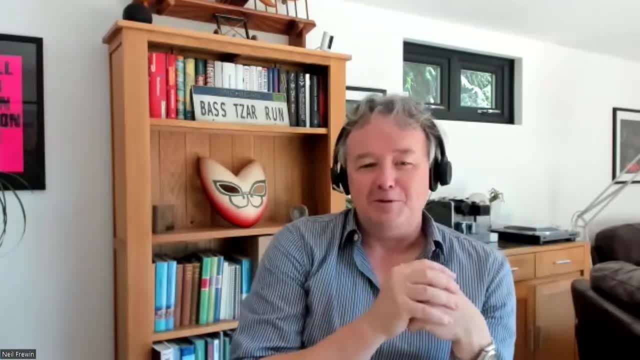 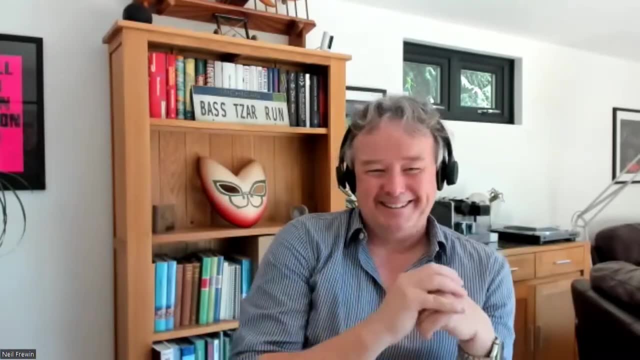 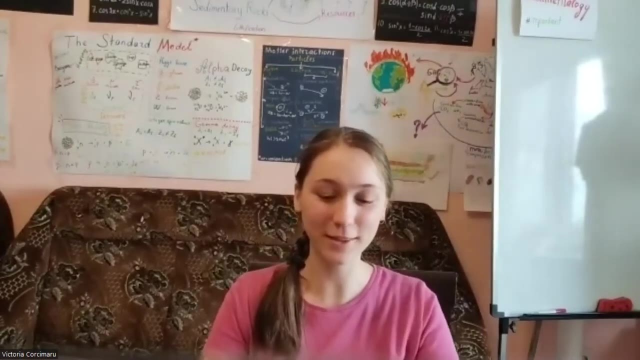 lovely. So I help out with fundraising and keeping the museum on track with a group of other trustees. So, yeah, that's me and my background and who I am. That is such a beautiful introduction. Thank you so much for that. And when you said when 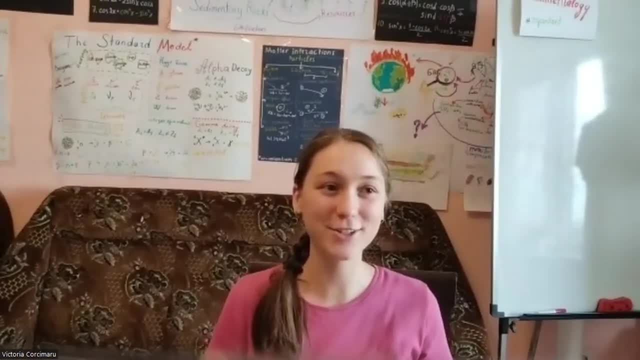 you mentioned the period of time that you've worked for Shell. it just dawned to me that you've been working in this very niche aspect of Shell for longer than I have even been alive. That makes me feel old, But no, you're right. unfortunately. 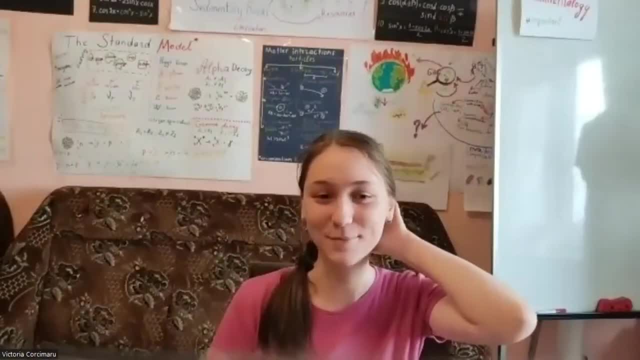 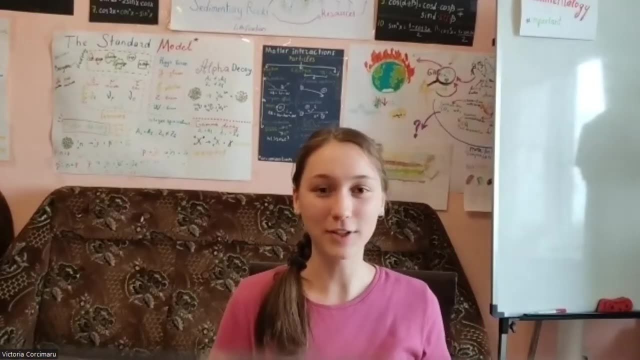 Yes, It makes me feel very unexperienced, But maybe that will help me ask questions that will at least reflect to some degree the general public of my age, which is an interesting thing, because we have a lot of contradicting messages being thrown around these days. 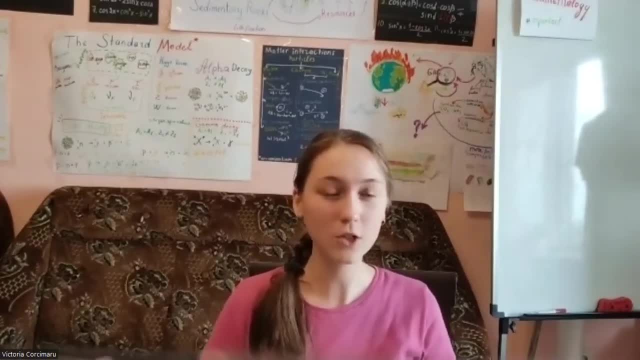 On the one hand, we hear about transition to newer energy sources, green energy and the need for that, And on the other hand, we hear about the need for green energy and the need for that, But at the same time, we hear of real world problems that cannot be currently fixed. other 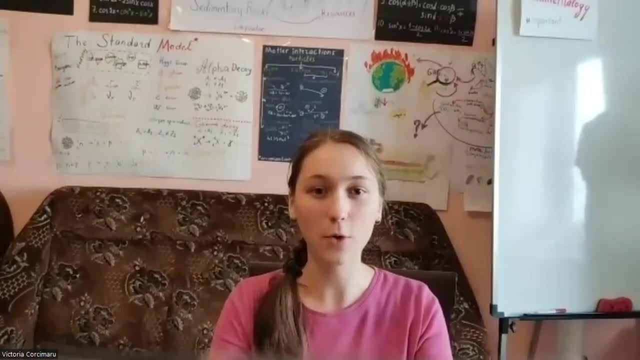 than by using the old infrastructure that we have, which is run on fossil fuels. And, having had this enormous experience in your field, I wonder how you can see the industry pivoting around those central issues, And I know this is a vague question, but I trust. 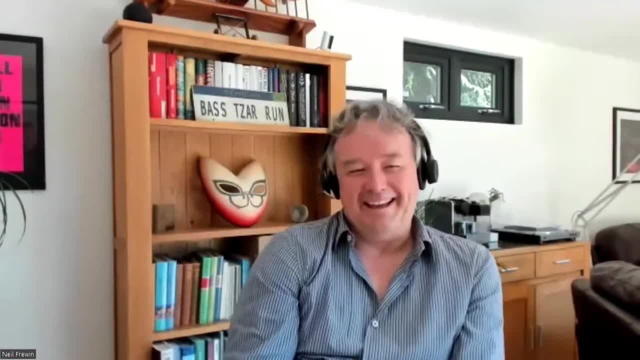 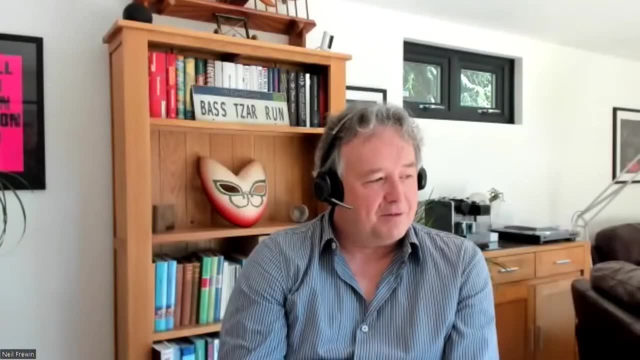 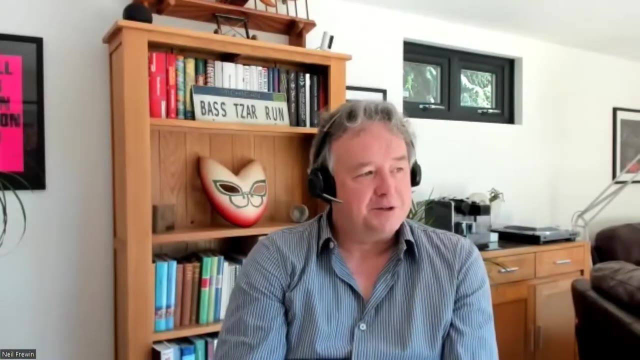 you to answer it. Thank you, Yeah, thank you. Well, I think you know society, certainly Western. let's, you know, be very careful about who we're talking about when we talk about different aspects of the transition, because, certainly you know, there are many societies on the planet, many countries. 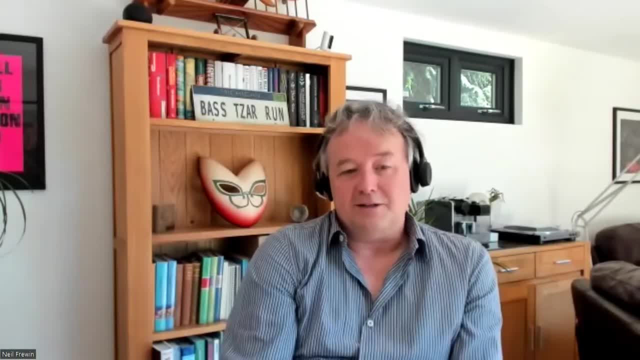 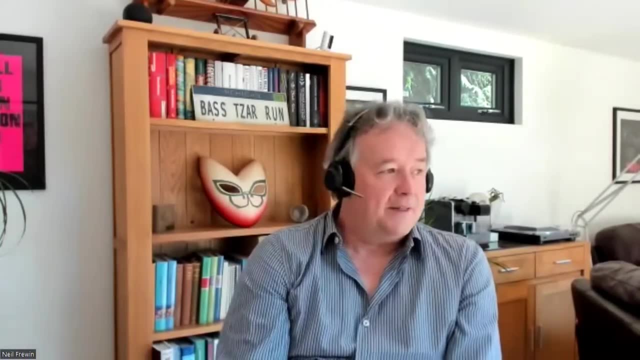 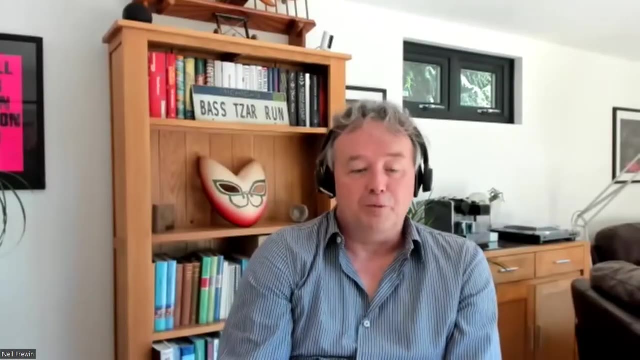 that have benefited hugely from. you know, oil and gas, fossil fuels and various resource bases have benefited in many ways. And then there are still, you know, countries and societies that are still growing through that at the moment and will still benefit from the resources the planet has. But I think 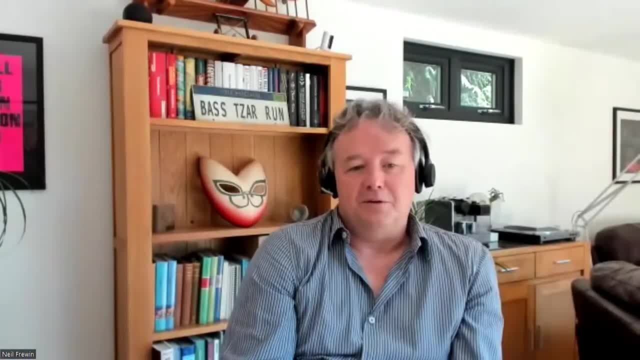 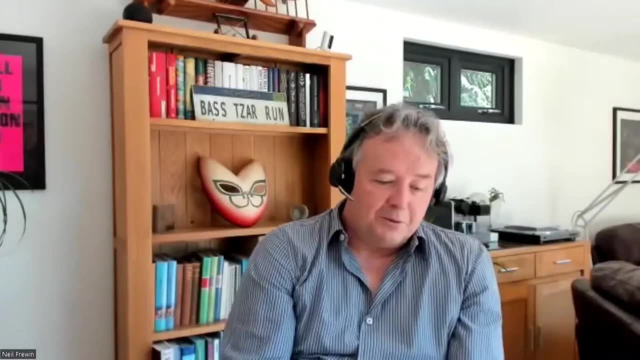 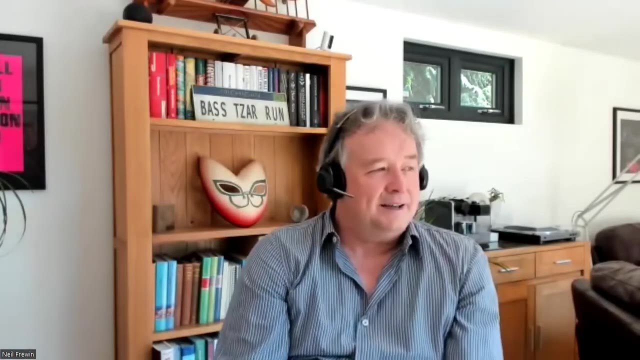 we all know that this isn't a very sustainable picture, right? So fossil fuels themselves are, by their very nature, a finite resource, And so you know, we really have to start considering that pivot tool through an energy transition, And I think the challenge is that's going to take time, of course, you know, in infrastructure, 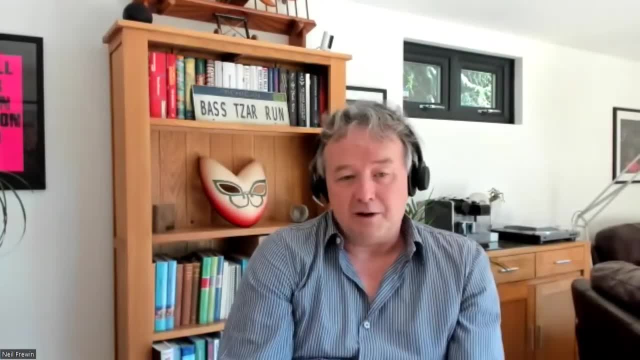 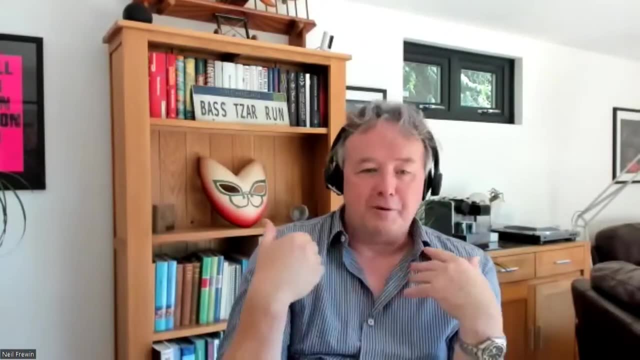 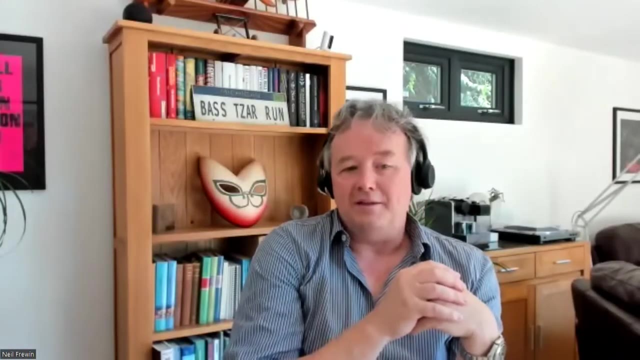 the infrastructure of most countries are very much based around the fossil fuels. in this country I'm sitting now in the UK, of course you know we went through the Industrial Revolution, you know, many, many decades ago and that's driven the way this country is built in many 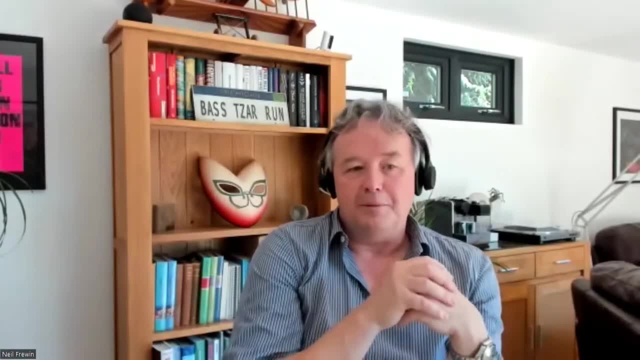 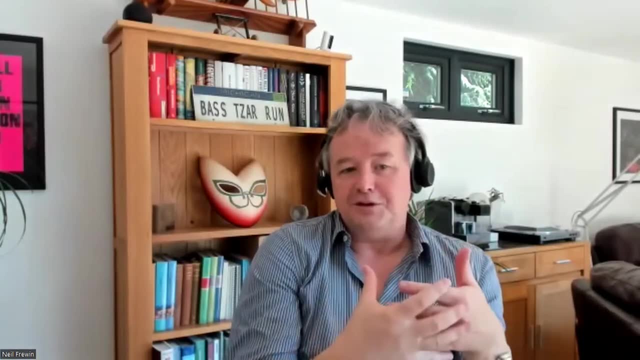 ways. So it's kind of hardwired into who we are. But I think you know, I think you know most. I think most governments are realizing that we're going to have to get through this addiction of oil and gas and move into something you know more sustainable. But what that? 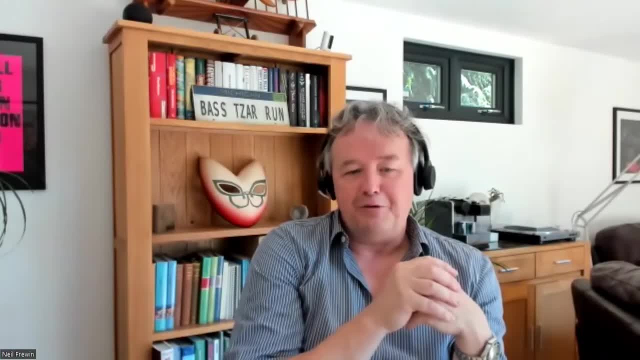 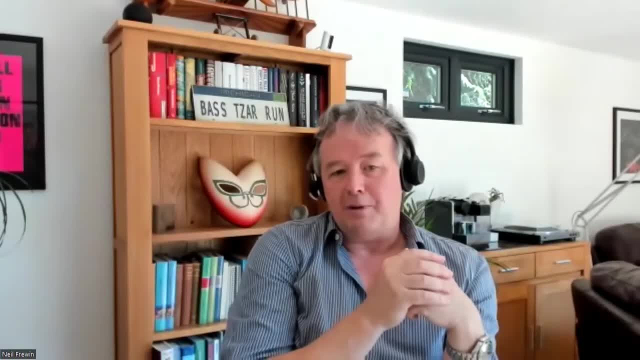 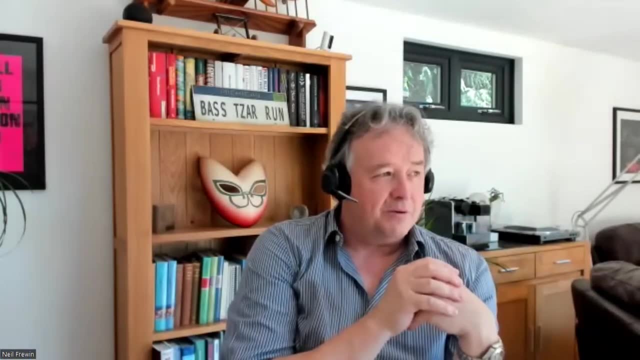 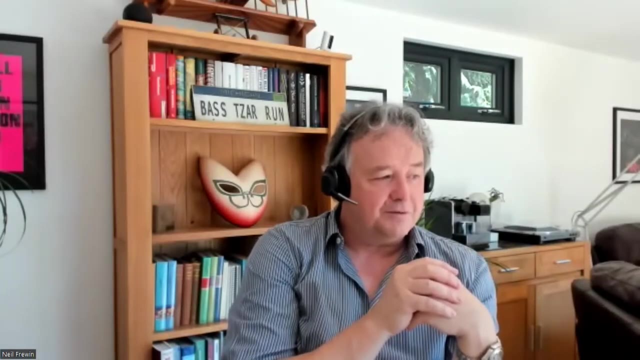 and can continue to power our planet and population that sits within it. So I see companies now really taking that seriously. I mean it's been interesting being in Shell, for example, for so long that I've seen this evolution over my entire career- lifetime actually. 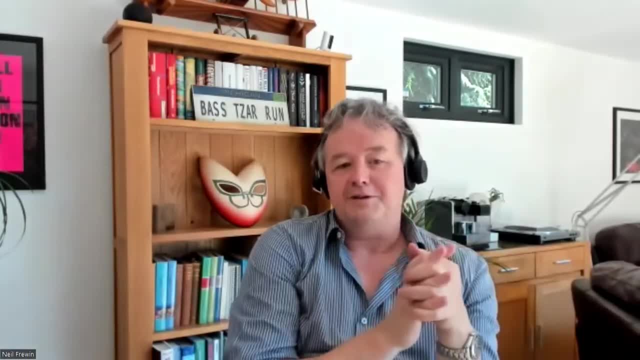 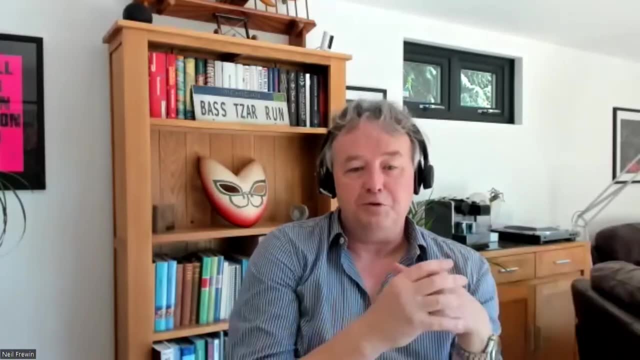 you know Shell's been in solar, we've been in hydrogen in the past. you know we've We've invested significant money- I wouldn't say as much money as we have done- into, of course, fossil fuels and hydrocarbons. 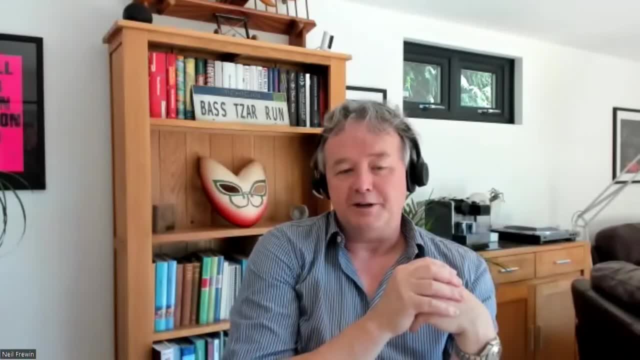 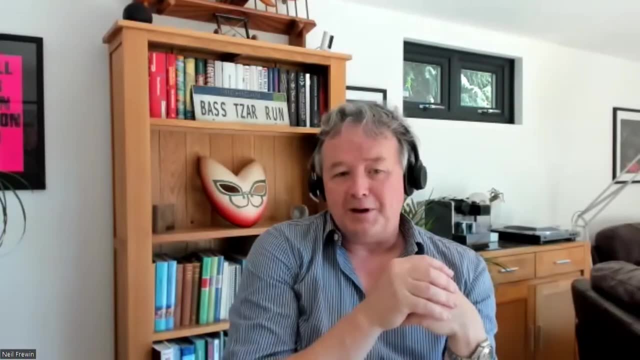 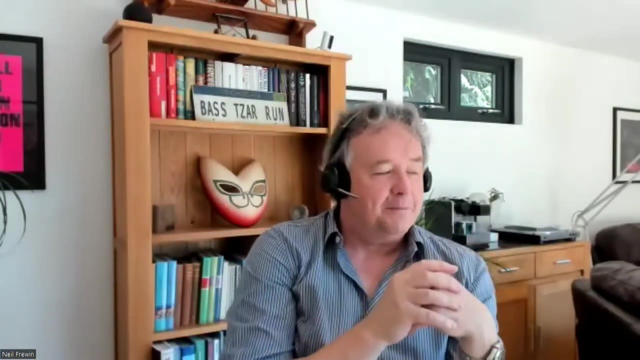 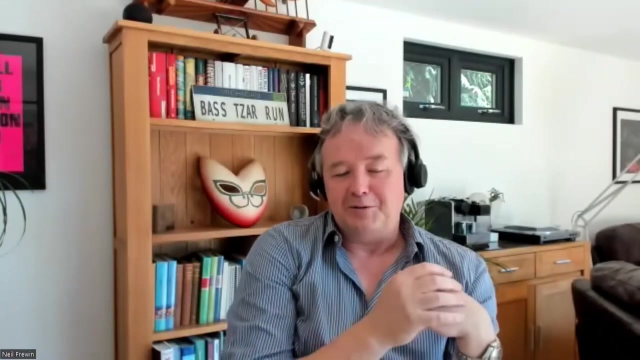 But we have invested significant money over the years into different aspects of more sustainable energy sources And those have sometimes come and gone if the economics don't add up, if the customer isn't interested, if it costs too much. But I feel now that this is the time where I think most of these companies are starting to really grasp the nettle and go after some of the fawniest issues of our future energy supply. 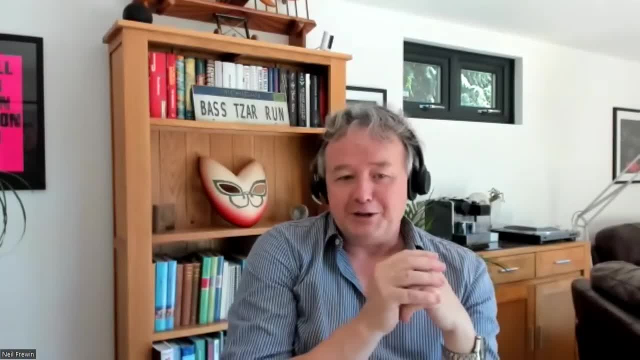 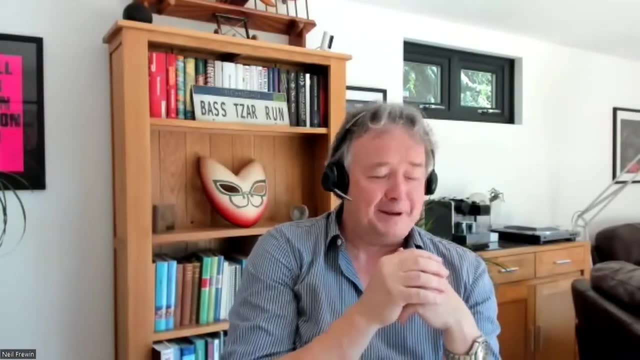 So I'm optimistic, but I'm also fairly realistic at some of the challenges that lie ahead And I do believe- and it may be unpopular, but I do believe- that oil and gas will certainly remain a part of that picture For some time to come. 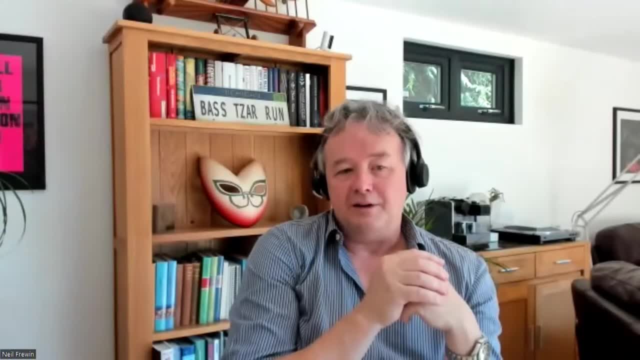 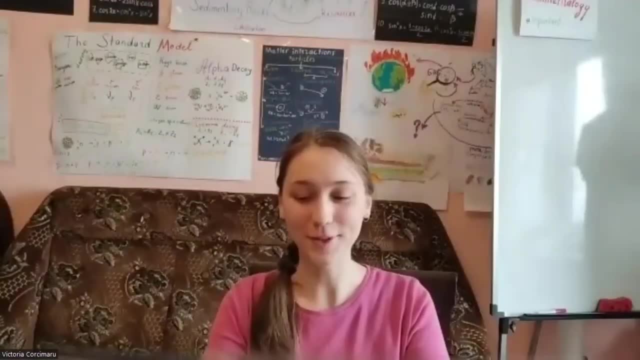 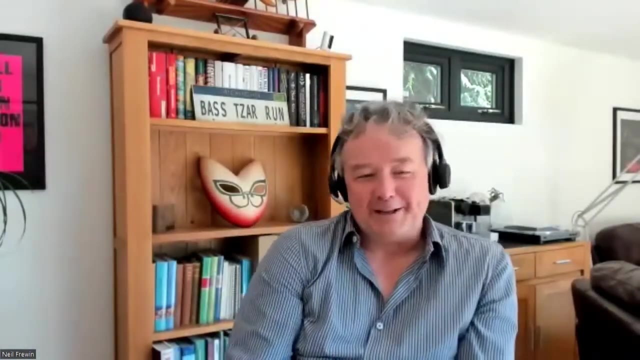 But we do have to start to reduce our reliance significantly on those energy sources one way or another. I couldn't have thought of a better answer. I hope that answers. It's a complex question and a complex answer, But I think you have to be optimistic and realistic. 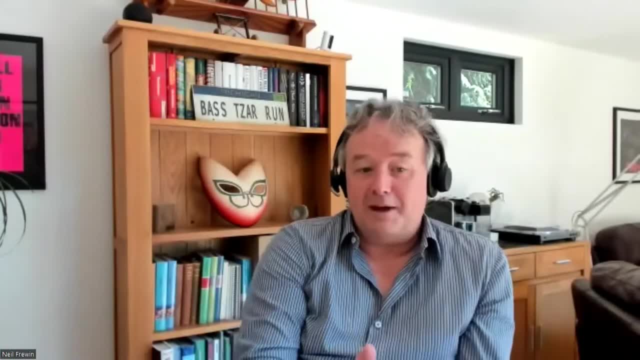 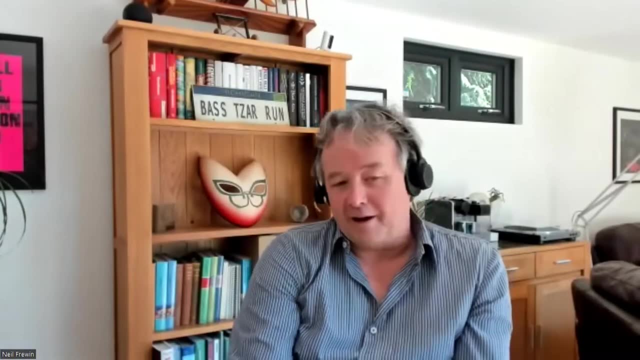 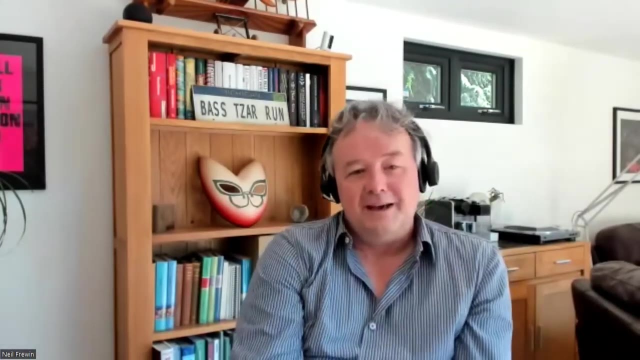 And I think we rely very much on people like you- you know who are our future- to really Think about the innovative possibilities that there are out there, And I guess we'll come to talking about skills and the skills that we require to do this later in the chat. 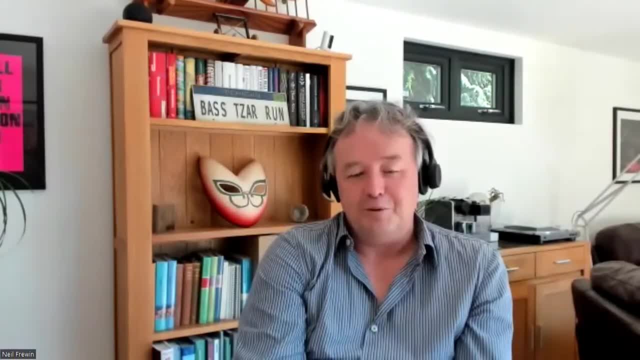 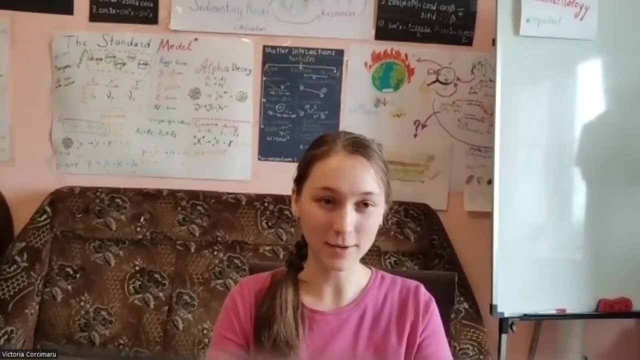 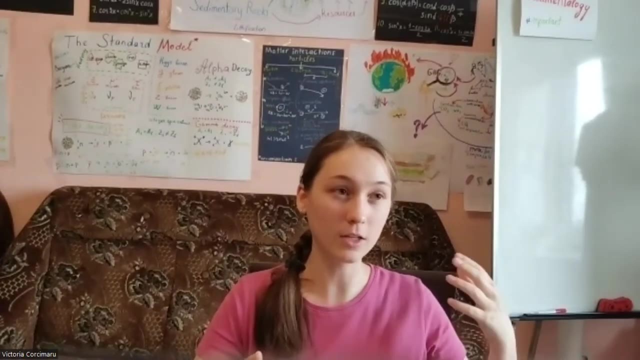 But yeah, I think it's really fundamental to moving forward. Yes, In fact, I was just thinking that, while we are on the subject of the future, many people in my time, at least in my generation- we think of fossil fuels and the enormous amount of energy. 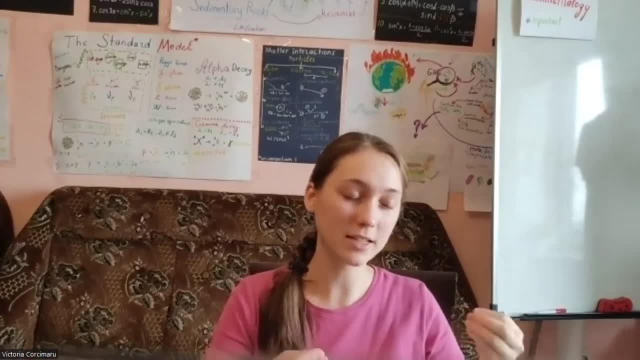 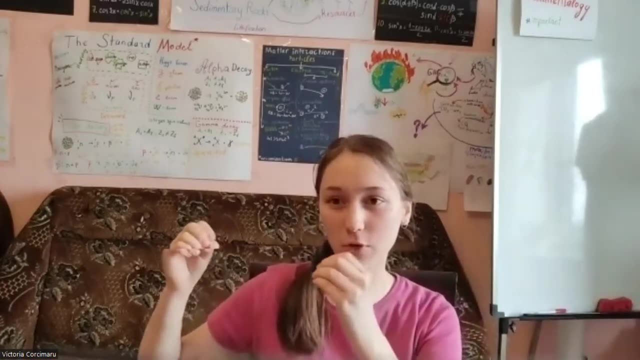 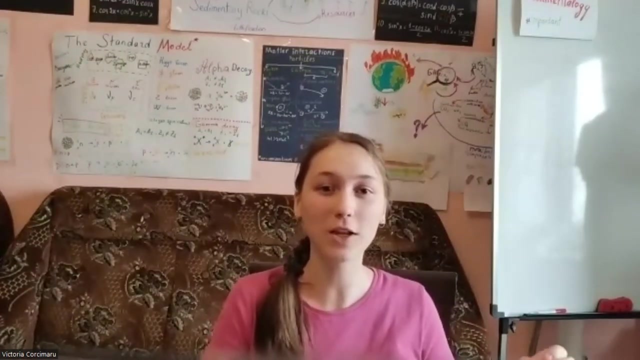 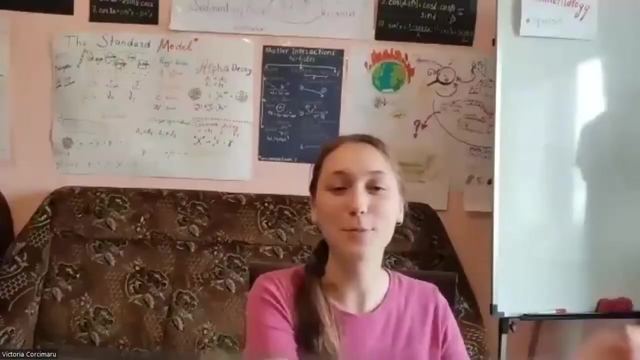 I mean mental energy and skills that were acquired by working in this industry have to just be abandoned, And then we move on to some sort of new knowledge, new science, And my question to you is: how can we? does this have to be the case, or can we reuse the energy, the knowledge from the oil and gas sector in a smarter way to move away from fossil fuel reliance? 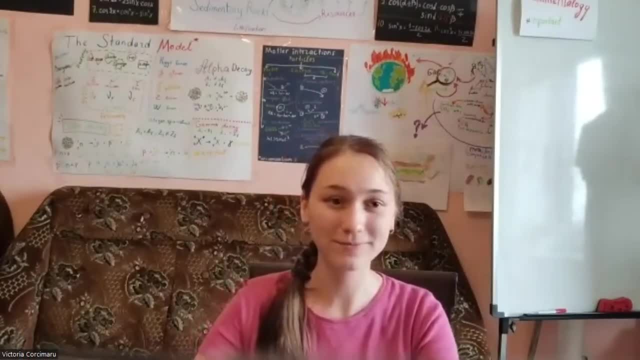 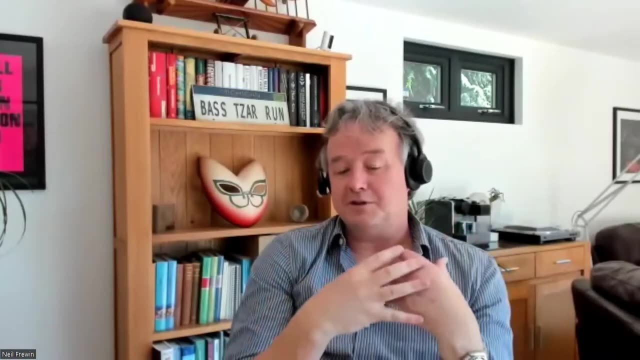 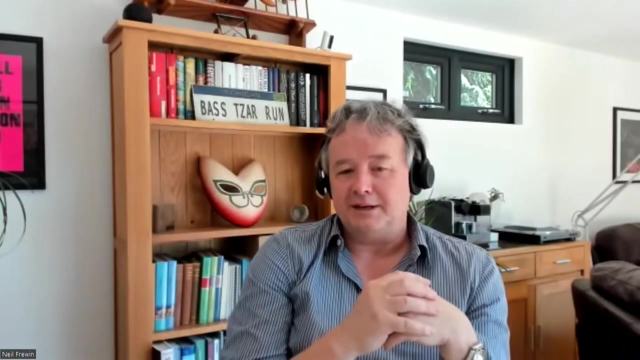 quicker than we will without this knowledge. Yeah, I mean so. the huge management of issues benefits, you know, understanding of the subsurface and of the Earth have hugely benefitted from the the the sheer amount of investment that oil and gas companies have put into understanding the subsurface. 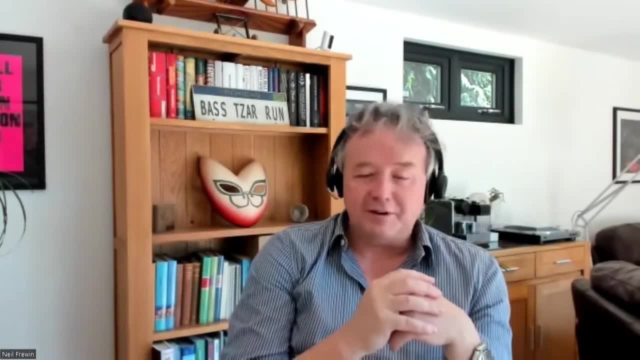 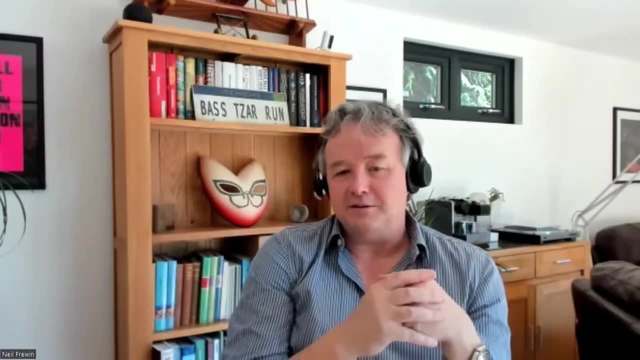 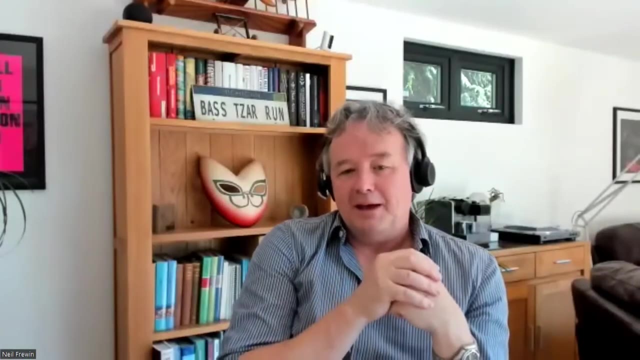 And both in terms of fundamental understanding of Of the way basins form of the subsurface, the uh of the way they're heated, of uh of the of the various depositional um systems that you see within basins, um, i mean, the amount of work that's gone into that has been huge. and then the 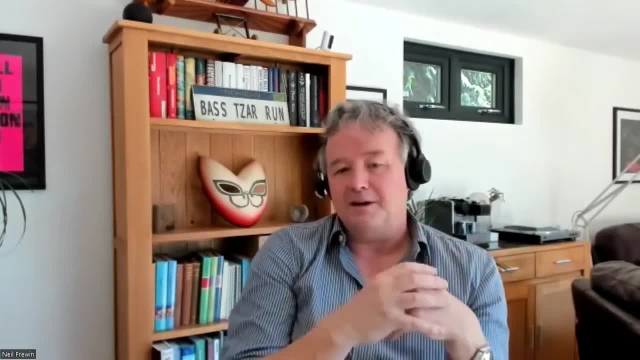 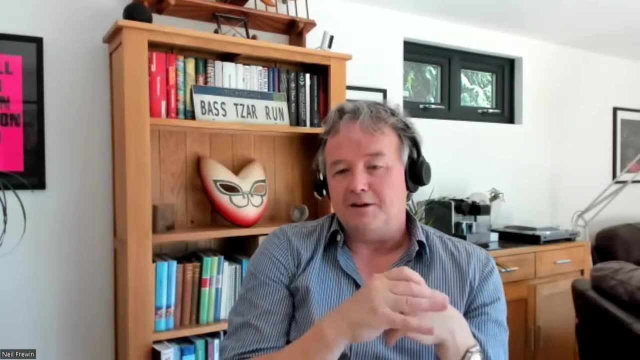 technology, technological development on top of that around seismic um uh, around imaging the subsurface and and really understanding it and visualizing it in detail, has been immense and uh, and i think that's something that the industry can be very proud of, actually, that we have achieved. 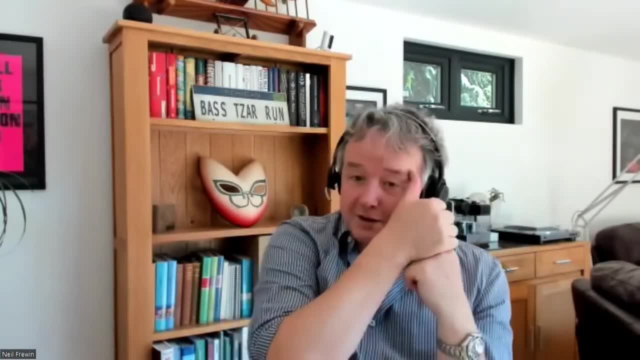 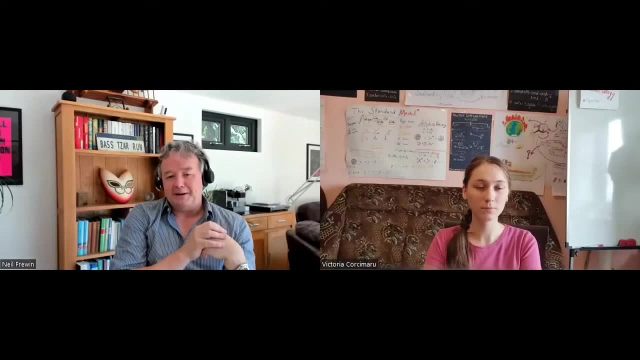 so much um over over a relatively short amount of time, um, in understanding what is, you know, the planet on which we all sit, and uh, and uh, and and live. so i think that's that's been really, really important. now it would be a shame to see all that thrown away, of course, and uh. 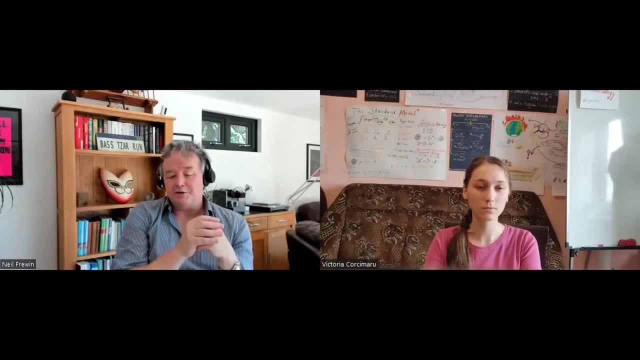 and i don't believe it has to be. i think there's so much that can be transferred now into various other um aspects of of the energy system. um, that will really create some benefits and um, uh, you know whether it's uh thinking about things like carbon capture and storage and 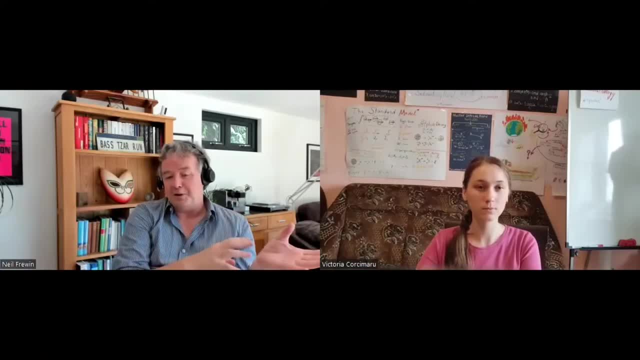 containment. um, you know there's plenty of work being done in oil and gas in terms of seals and containment and barriers. um, that directly link, of course, into into understanding how you can contain and store uh, carbon dioxide, or even, you know, hydrogen as an energy source. there's, there's. 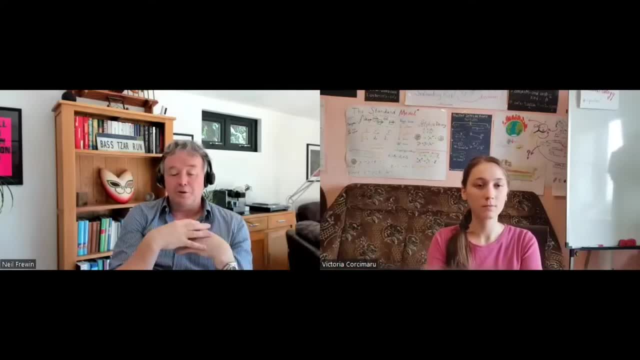 a lot of work around that um, you know, a lot of the forward the earth modeling that we've we've developed over the over the decades. there's there's a lot of um, a lot of transfer there as well. uh, we're already using a lot of our basal modeling tools, for example, in the geothermal 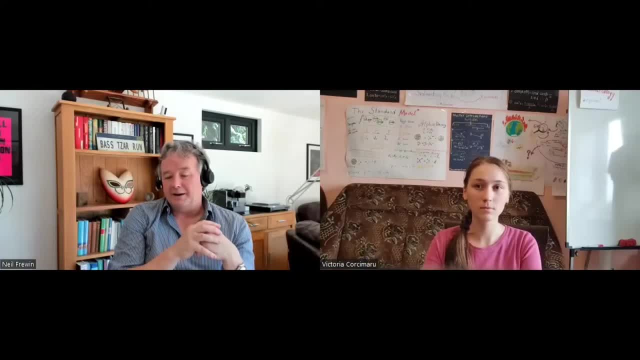 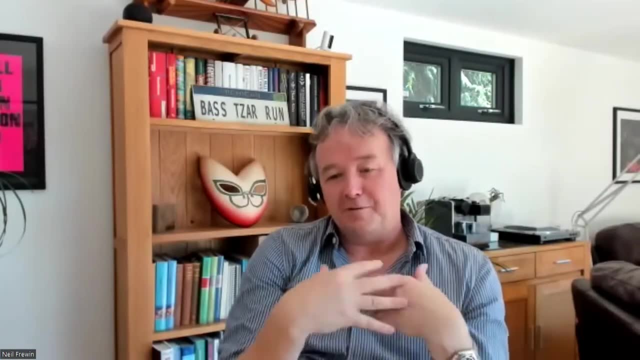 realm, realm. so looking at um, uh, uh, you know heat in basins is very much something that uh, that uh, the uh, the petroleum geologists do all the time. so you know it relates directly into geothermal applications, um, seismic and shallow geophysics, you know. when it comes to wind farm, 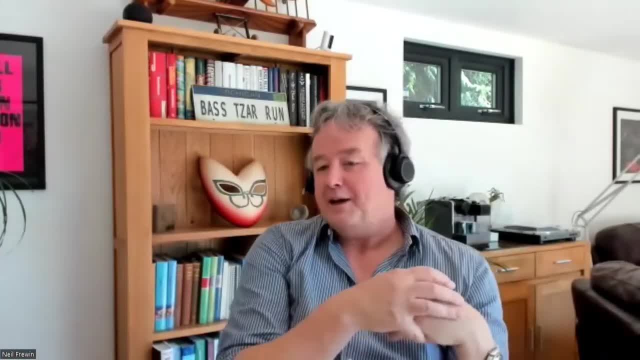 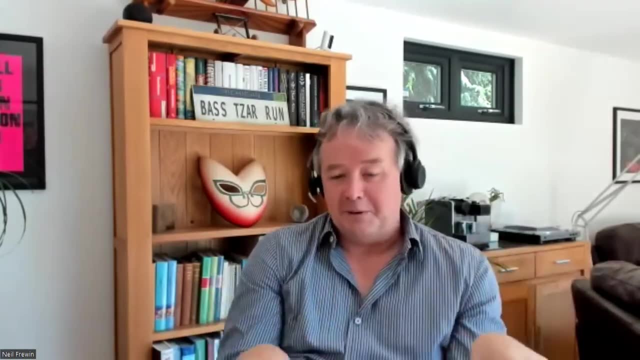 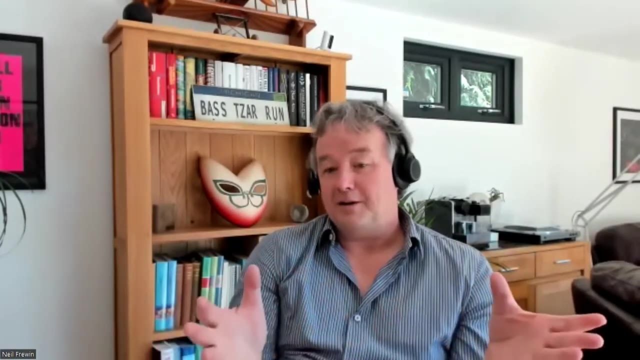 siting, drilling hazards, shallow infrastructure- there's a lot of work that's been done there as well, um, and then finally, of course, there's so much data, um, about the subsurface. now that you know, the whole digitalization process will allow us to create, i think, uh, with enough work and enough investment. 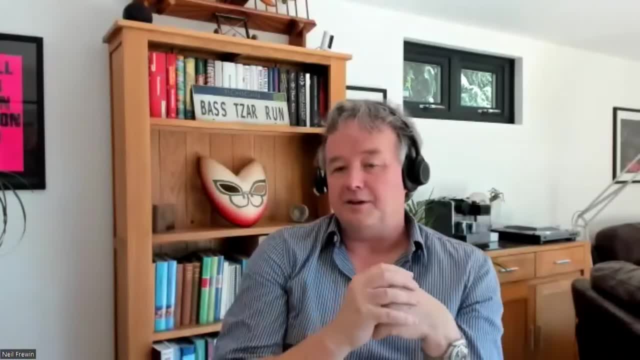 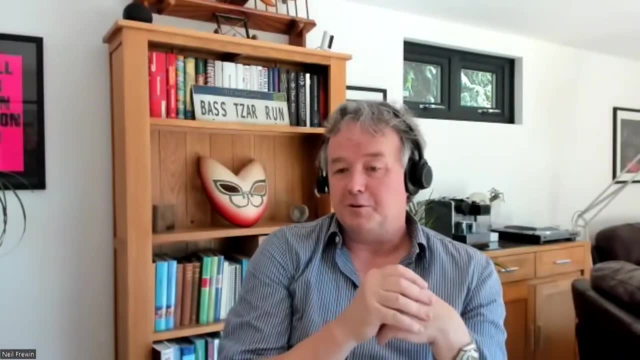 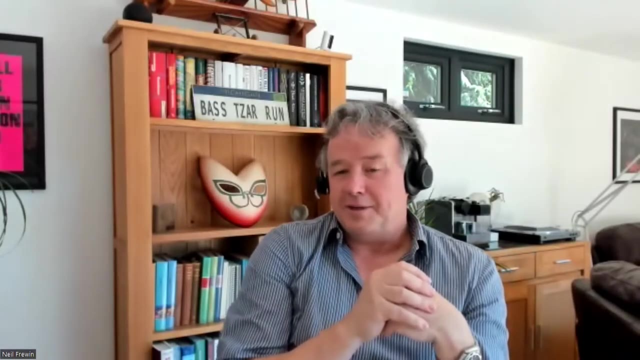 continued investment, a very digital earth and, uh, that will allow us to do so much more, i think, in terms of, uh, in terms of understanding the earth as a resource, but also, uh, you know, as a way of sustaining, uh, you know, the, the energy resources that we use and build on. so so i think, 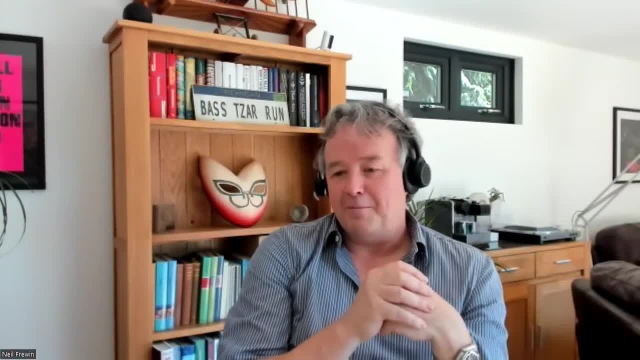 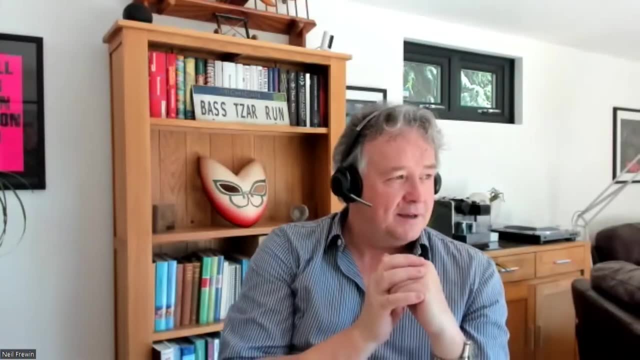 there's, there's a huge amount that can be transferred and, uh, you know, i'm i'm very optimistic that that's, uh, that's out there. in fact, we have a conference next year, um which we're putting together at the moment in uh in aberdeen in scotland, um which will really be looking at uh. 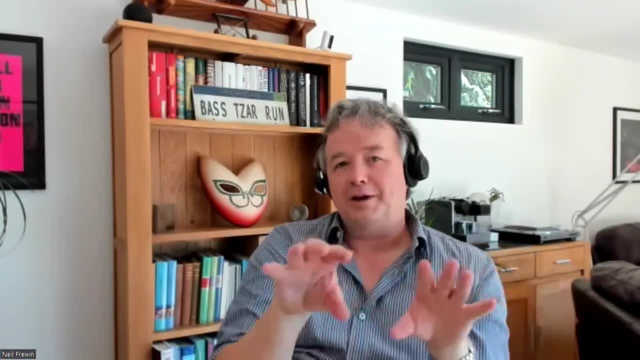 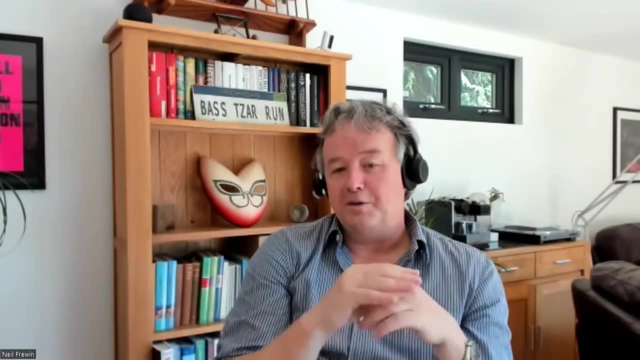 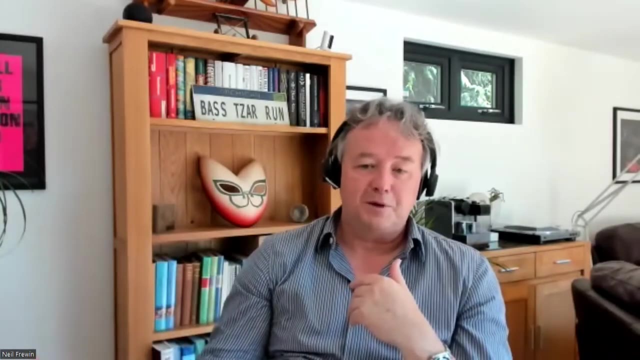 geoscience practices, uh kind of agnostic application, agnostic to, to, to where they've gone. so so taking a look at all of these methods that uh, the petroleum geoscientists have used in and then applying them to things like, uh you know, nuclear waste disposal or ccs or wind farm geology. 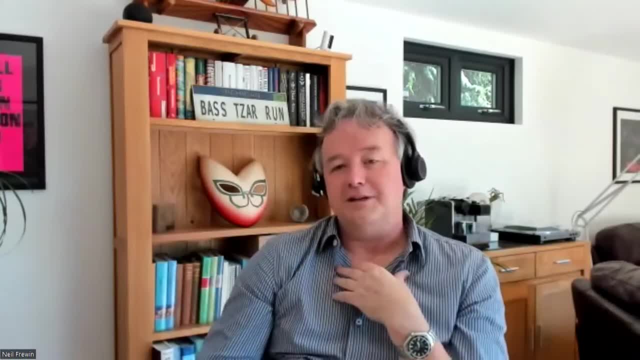 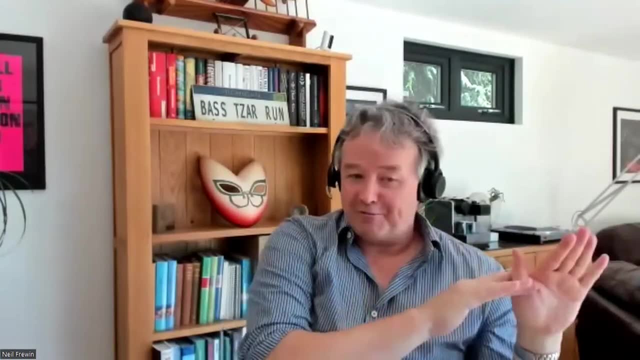 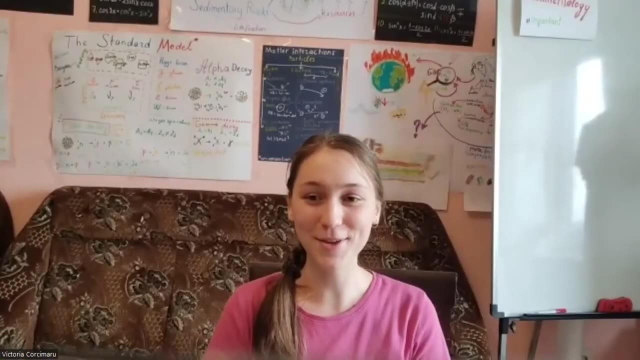 or geothermal, really applying it across those different, uh, different areas. so, uh, there's plenty for geoscientists to do. still, lots of skills still required and a lot, a very nice foundation on which we can build further. wow, that's impressive. that makes me so excited, just. 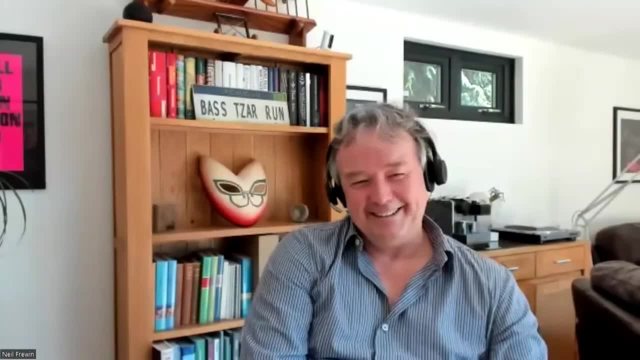 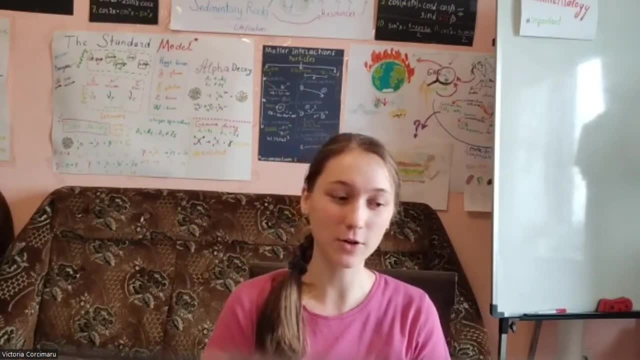 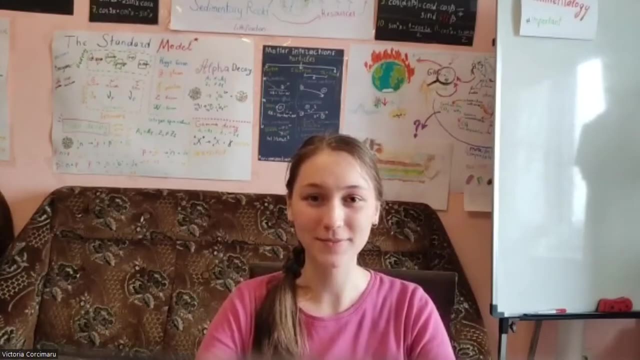 listening to that answer because it really makes me feel like there's a lot to learn and all of it is necessary and you don't have to have this fear of if you learn something today, maybe you will go out of date or out of fashion the next year. so, yeah, i think it's all still applicable and you 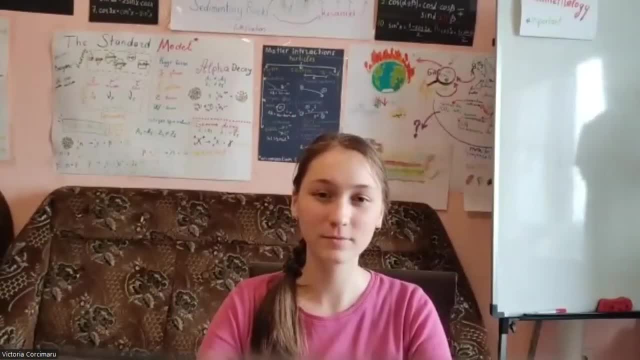 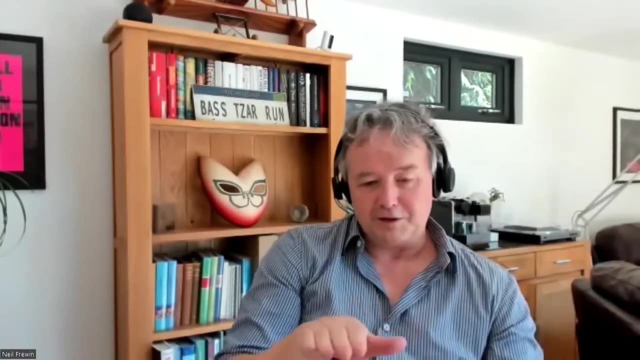 know at the moment in shell, we're, you know, especially in my area of, of, of, of focus in specialist geology, we're looking at how we kind of reorder those skills to to apply to different parts of the business now. so, uh, so carbon capture and storage is a big. 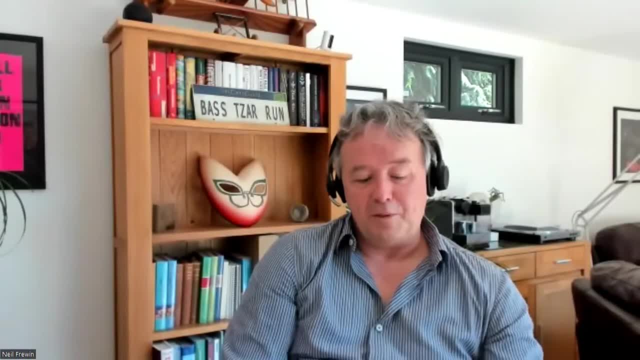 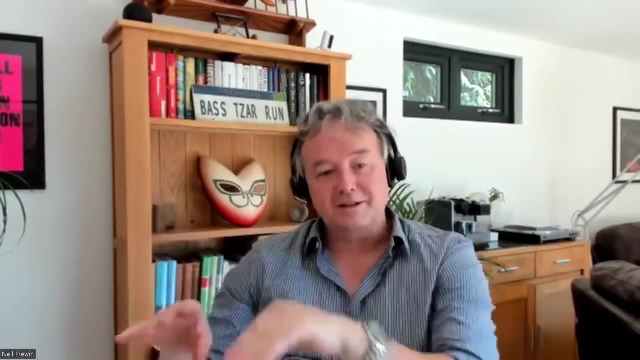 one, of course, and uh, and suddenly you know the things we might apply in the petroleum realm, we might apply differently in a carbon capture and storage realm, but but actually the skills slightly in a slightly different order, um. so so piecing that together is quite exciting actually. 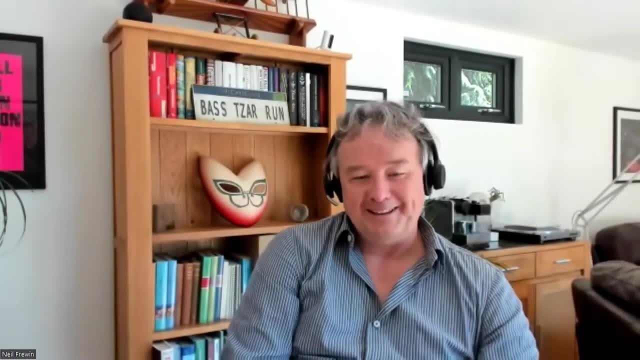 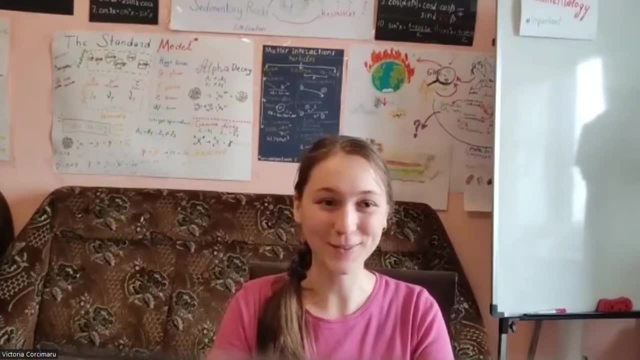 and i think, uh, yeah, there's plenty to do there for sure. it's a great moment to move on and ask you about your actual work at shell. so what is your actual work at shell and what is your actual work like? what do you do? yeah, so my day-to-day work now is: uh, is so i'm a geochemist, as i say by. 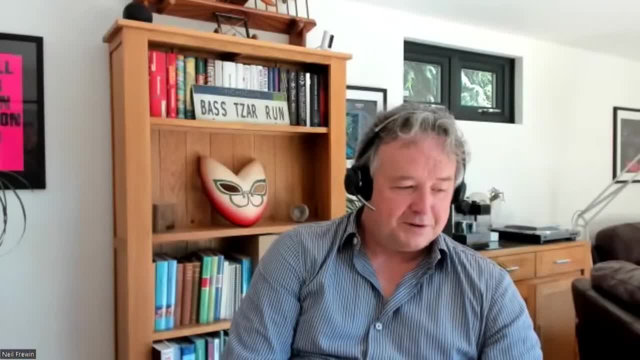 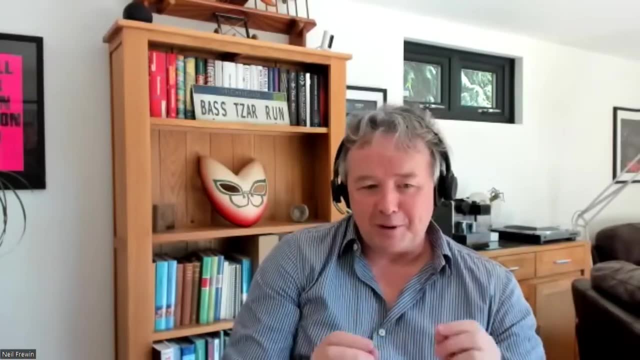 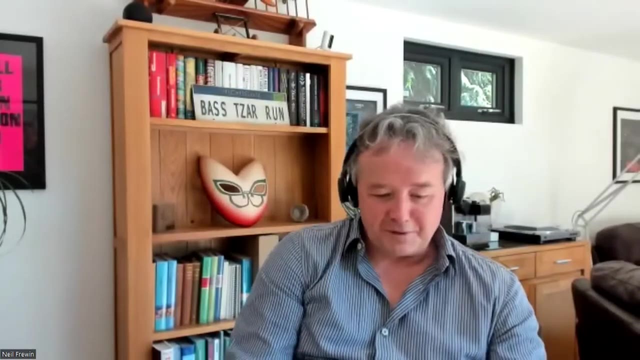 background and uh, you know, i've, um, i've worked at a molecular scale, uh, for for much of my early career and my phd was at a, you know, pulling together, pulling apart rocks and looking at organic matter. that was uh, that was uh contained in there, and uh, and trying to work out from this. 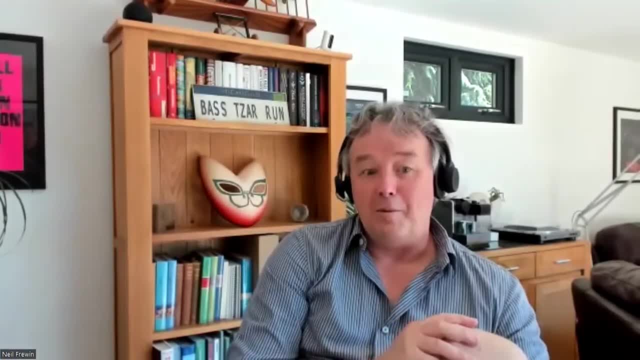 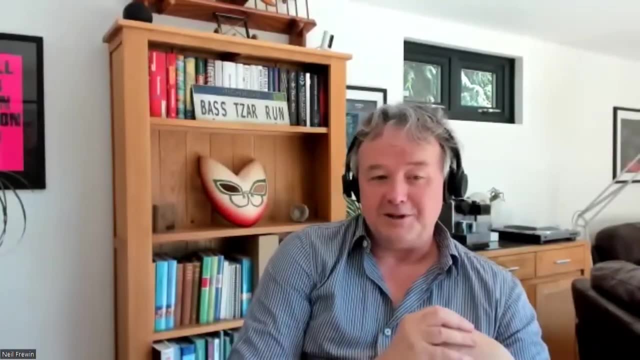 sort of these carbon, carbon structures. you know what plants they may have come from, what they may have been, and so i've been working on that for a long time and i've been working on the organic assemblage at that time. so so i still apply that now in some of my technical work, which 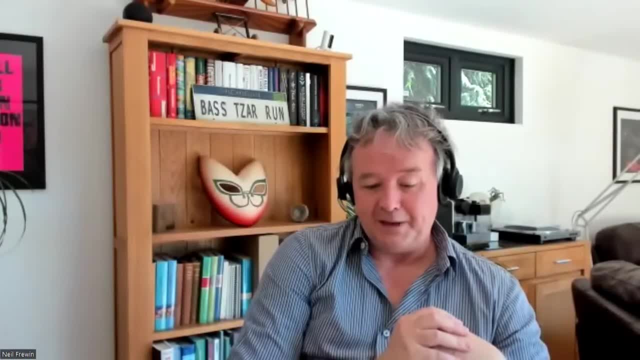 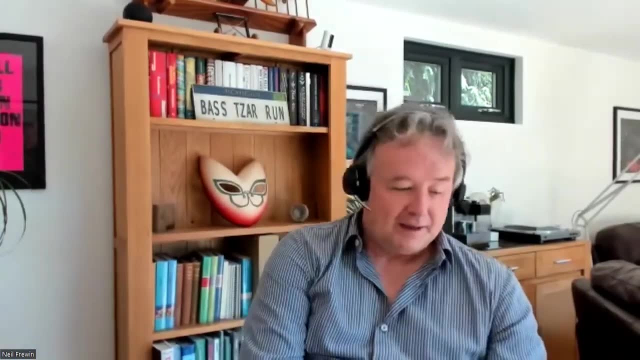 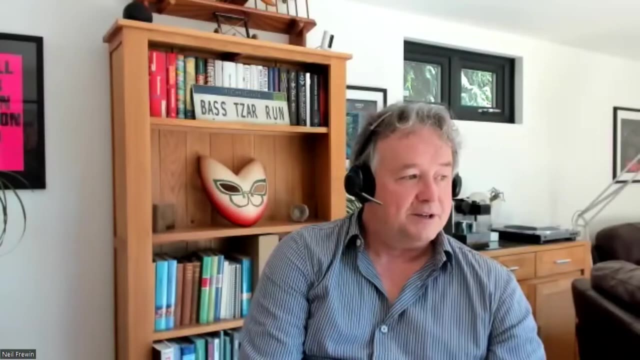 i i do you know, with the various projects um and uh, and apart from that, i'm coordinating a team that do very similar things with their own specialist disciplines- um, uh. prior to that, i've worked in in new ventures, uh, for most recent years and that's really around uh, screening, uh of basins. 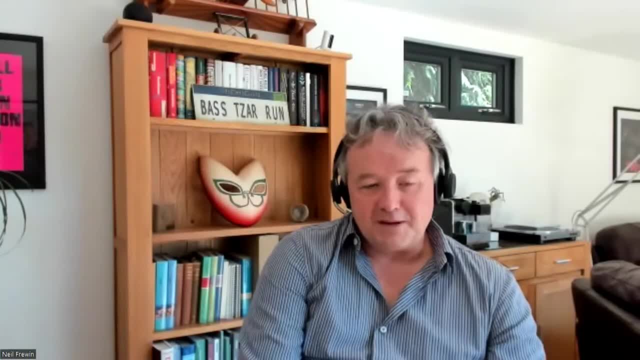 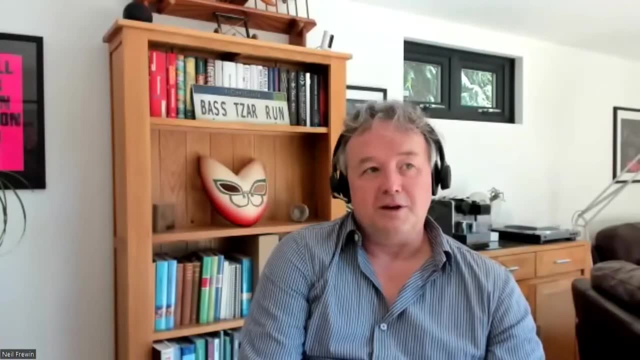 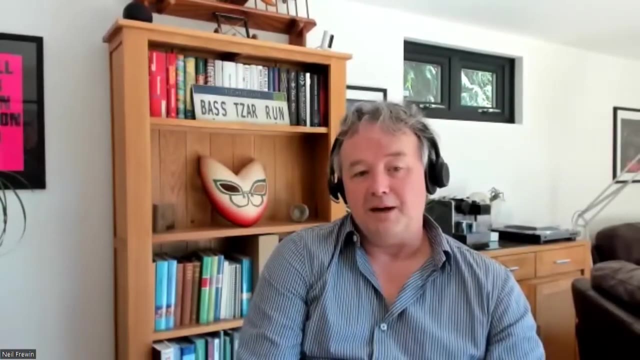 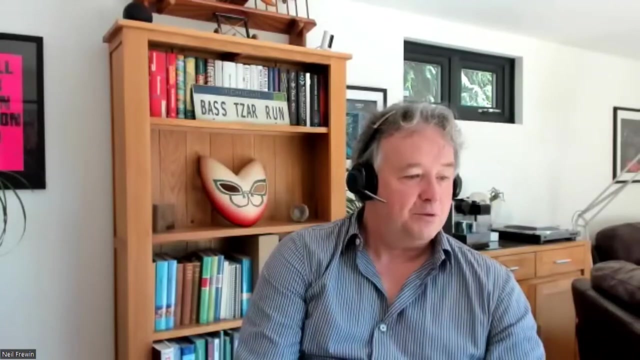 globally and trying to understand, uh, whether those basins will uh will be prospective for oil and gas and uh whether that's whether those are countries um and basins. we want to enter as a company, um and really start up a complete new venture um, and of course, that comes with quite a lot of uh consequence as well, um, because when you know a 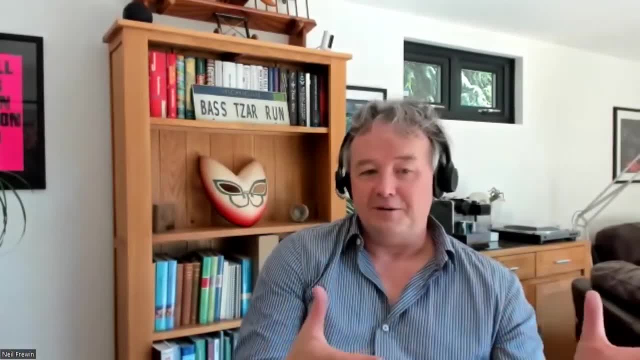 company like shell enters a country, you know it's, the brand is so significant that, so that that is quite a big move for the company. so, um, i've been working on that for a long time and i've been working on that for 10 or so decades and i've been out of oil. 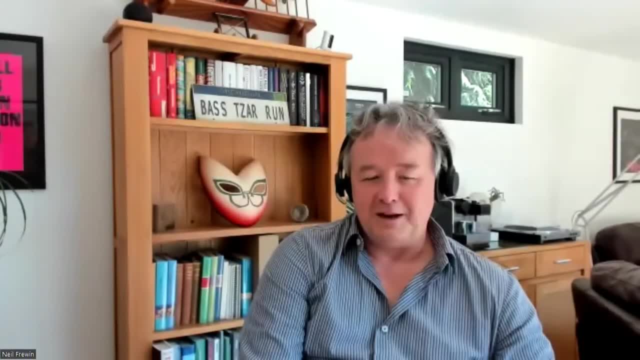 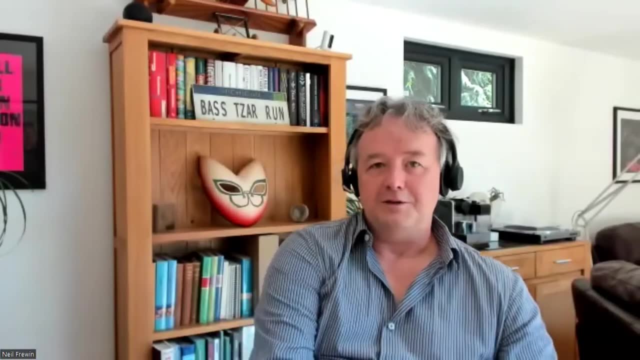 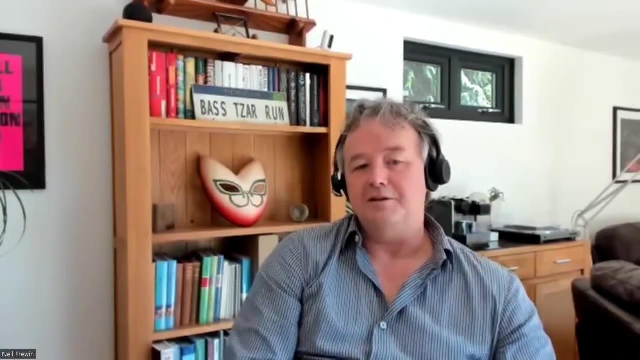 So you really have to be sure what you're doing. you really have to have really understood very, very carefully what the consequences of your actions are, um, how that will relate to the population, how it relates to the environment, um, and do you really have a commercially viable venture at the end of? 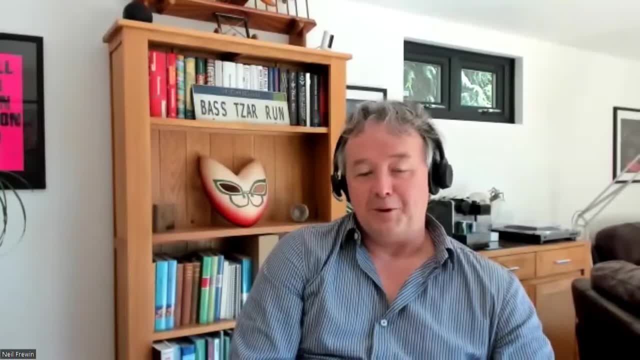 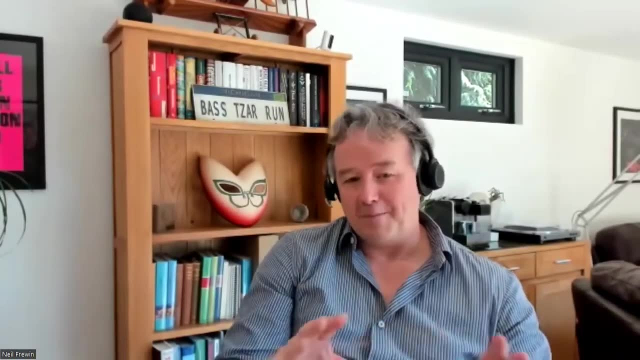 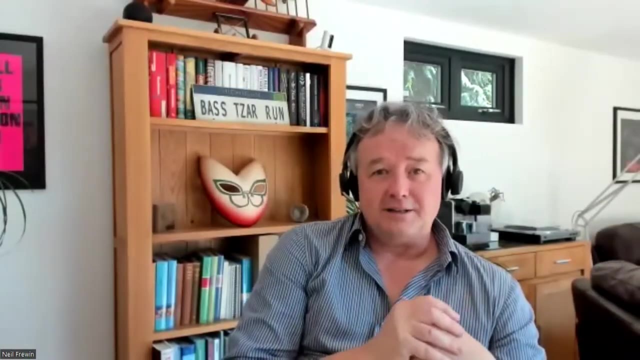 the day. so so to do that it requires, you know, a good understanding of the subsurface, but also a very, very good understanding of the surface and, uh, the commercial environment and the environmental environment. and you know the, the, the, the environmental environment and the environmental governmental environment. so all of those things play a very significant role. um, and that's and 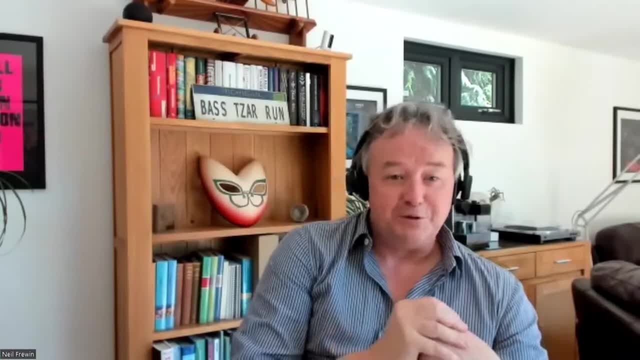 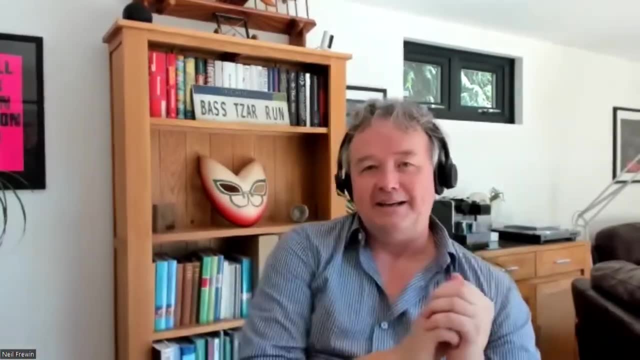 it's. it's a very exciting job to be in that. it's quite, it's quite stressful, it's quite uh, it's quite nerve-wracking sometimes, uh. sometimes you can be speaking to a government, sometimes you're speaking to a university, uh, or sometimes i could be sitting. i've once or twice been sat, you know. 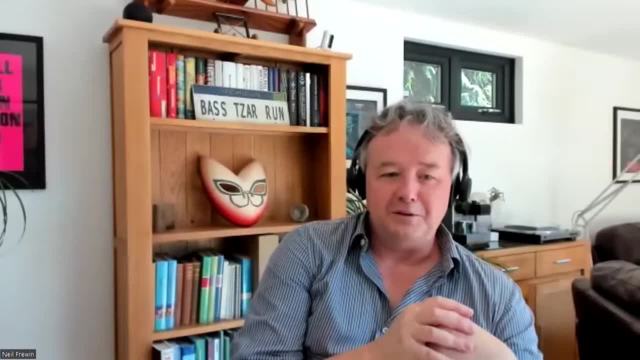 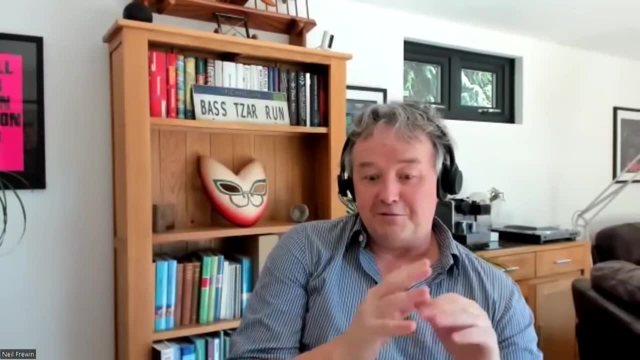 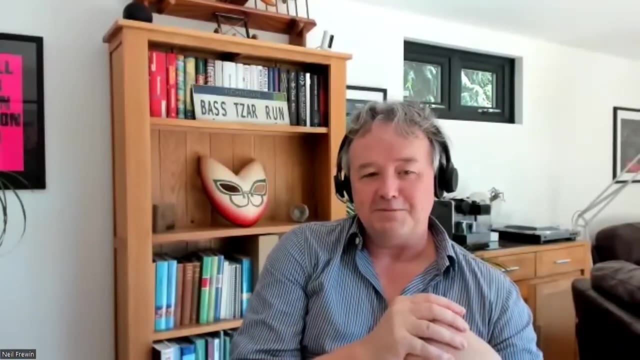 on a park bench, uh, in a field, talking to someone from the world wildlife fund, for example, or from a from a local conservation group, um, and so the variety of interactions you have in order to get to a sort of balanced decision on whether you enter a country is, uh, is. it's complex but fun. 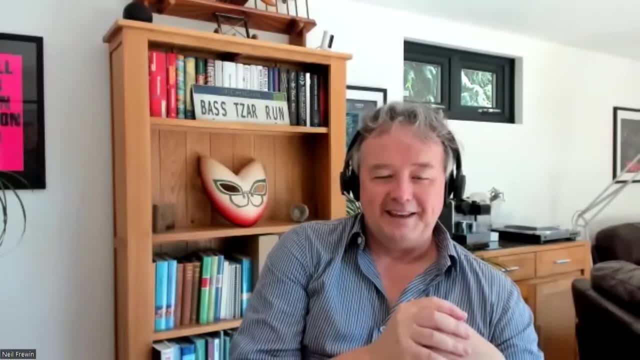 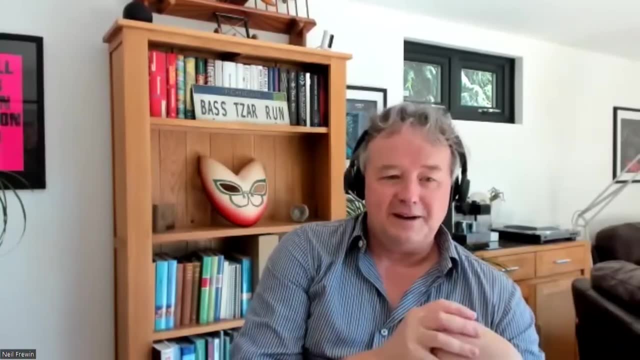 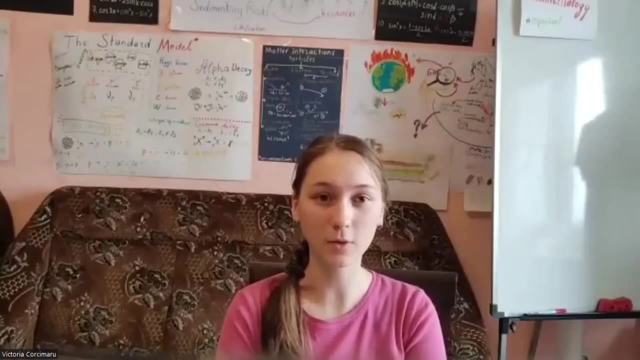 it's, it's it's a good thing to do, and you always try and do the right thing. i mean, it's really about doing the right thing, um, uh, commercially, but also, uh, environmentally and uh, and for the people that you're going to be interacting with. yeah, of course, and it's probably getting only 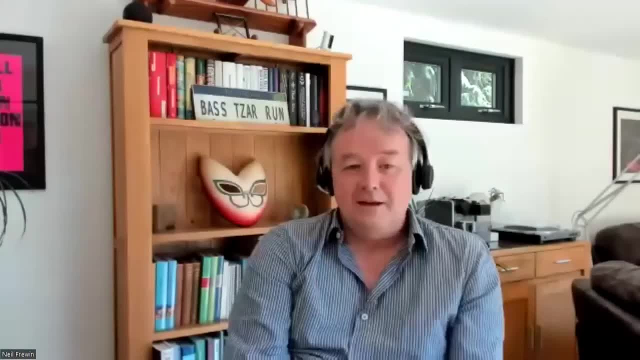 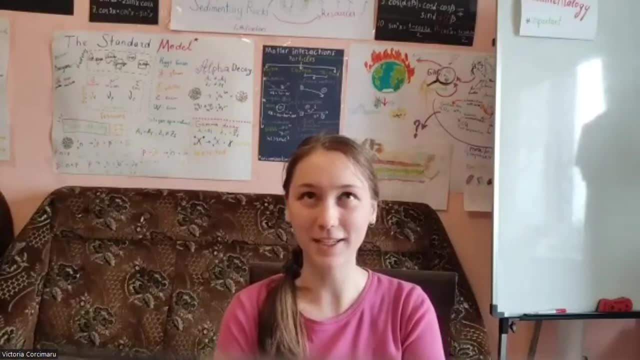 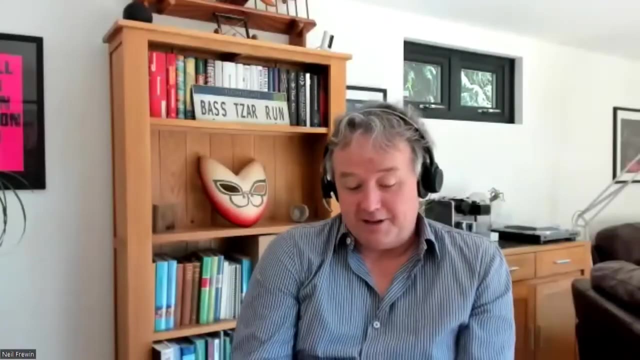 more, more and more difficult to do, because you have to drill deeper and have much more data sampling and analysis before you decide on whether it's worth it or not. is that so? yeah, yeah, it's become more challenging over the years, actually. and, um, you know there was a time when, uh, you know you feel like really an explorer- right, you'd be the. 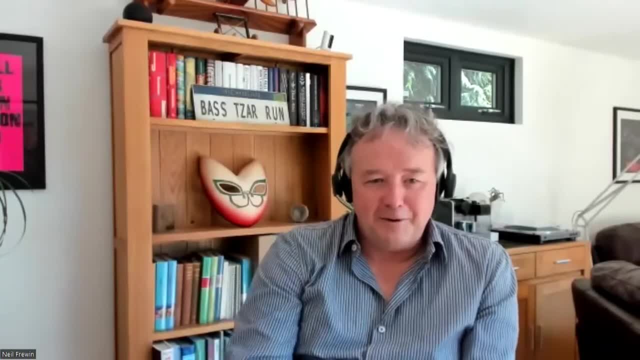 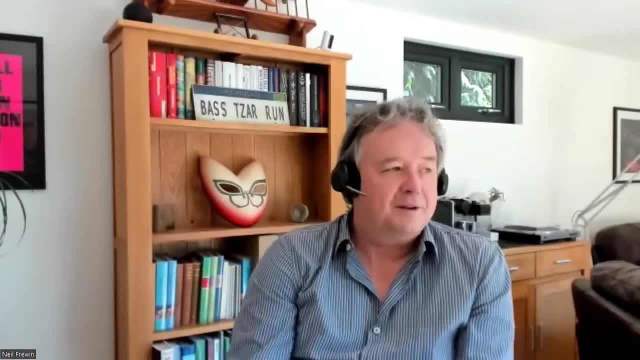 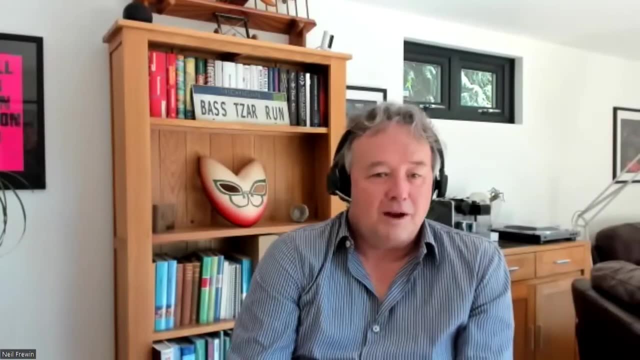 and to really look at that subsurface, uh, that part of the world, um, but now, of course, the world is very well known, the you know, a lot of the basins around the globe are very, very well explored, are very well understood, um, and so often now it's: you know, your, your exploration is back. 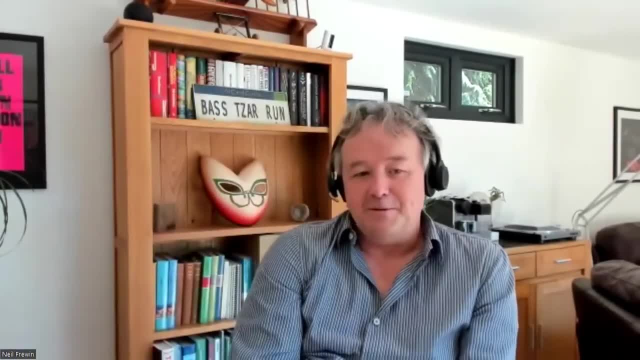 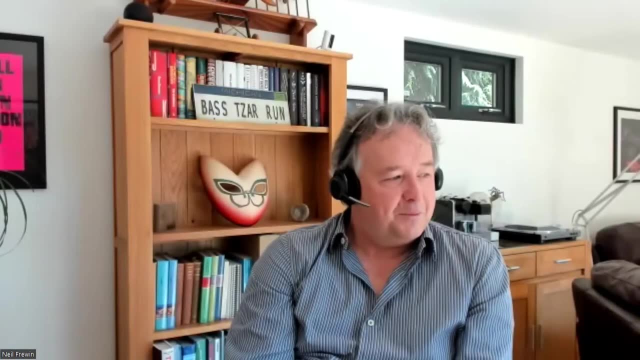 through data. you may have looked at 20 times before um, but you can look at it with new eyes, you look at creatively, you look at it with um, uh, with, with a sense of, of new thinking. you know what else could, what are, what other possibilities are there within the data that? 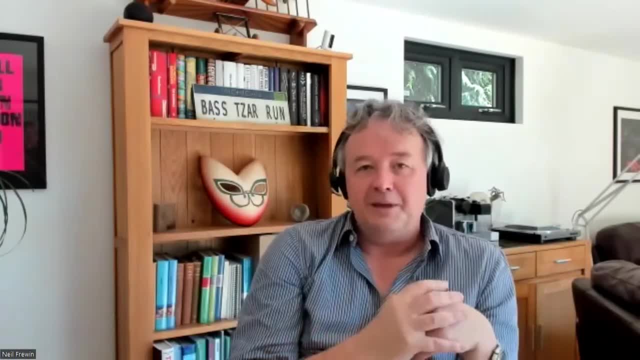 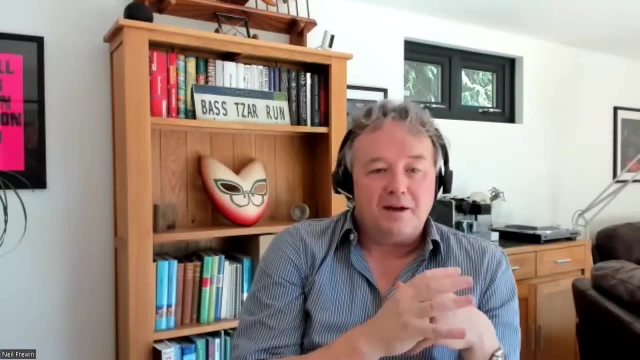 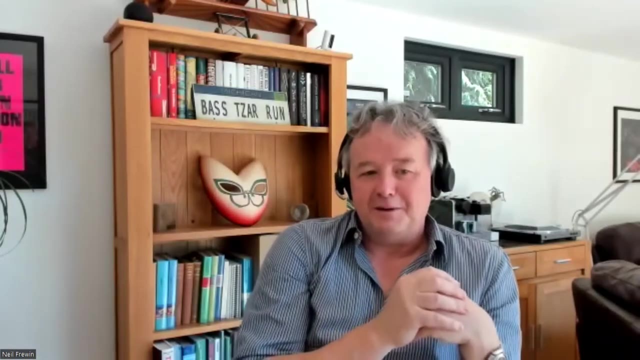 i've seen that that creates something new. um, so it's, it's. it's changed dramatically, i would say, since i started the industry to now, as to how we go about doing that kind of screening, uh, globally. um, i must say i did. i did like the kind of romantic early days of being the explorer. 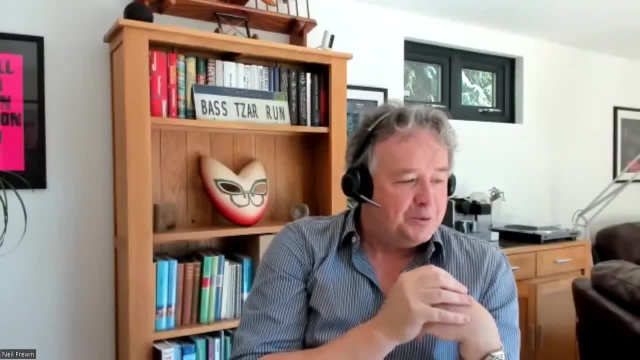 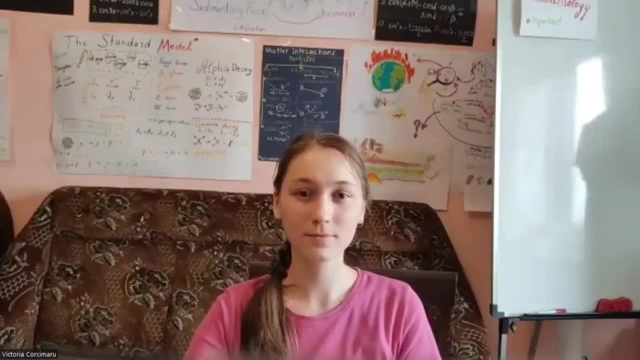 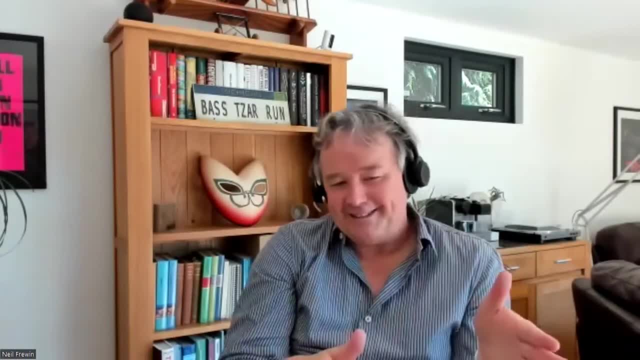 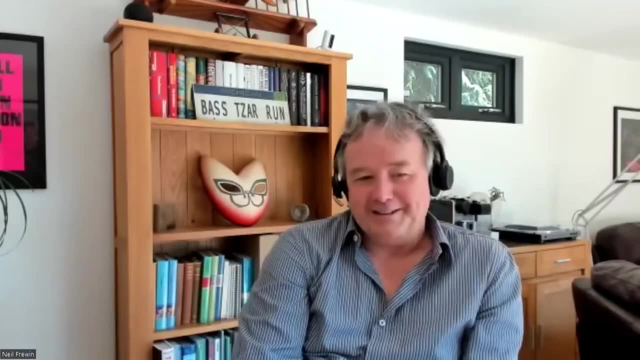 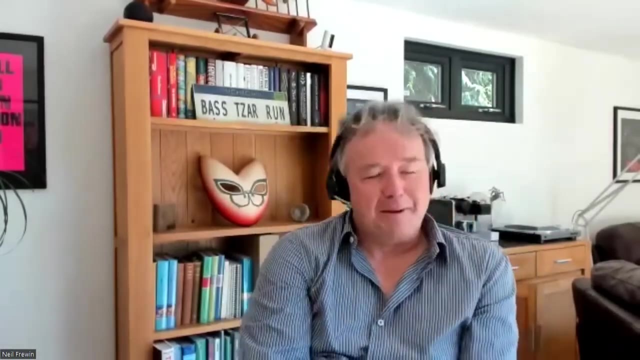 uh, looking at surface geology and thinking, how does that relate to what's going on under the ground in a relatively poorly explored area? and uh, and that's exciting, that's what keeps me, keeps me going and keeps me interested, are those kind of things. but but nowadays it's becoming 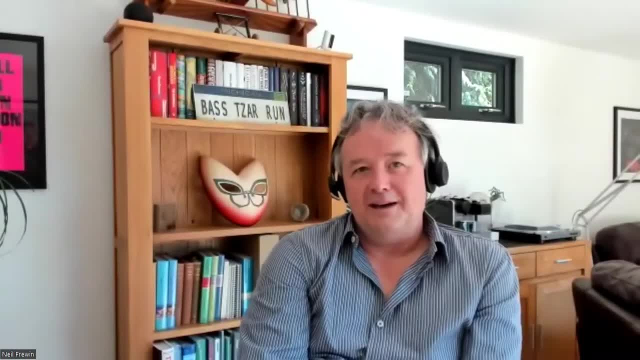 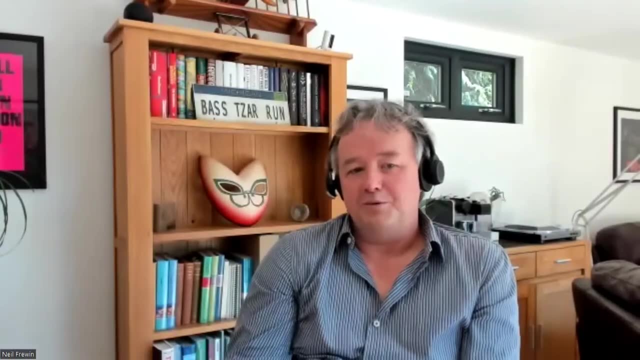 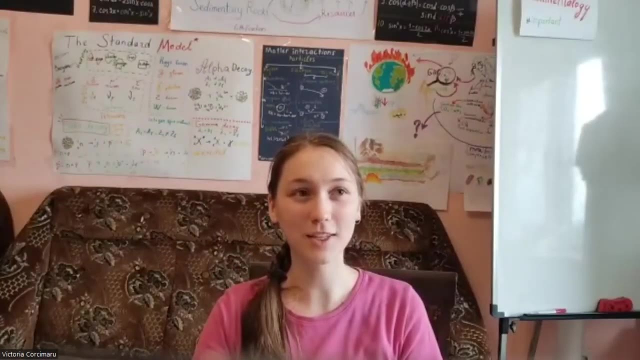 more about data and and how you look at data, how you uh integrate data uh from different sources, and and how you can build uh a picture of what else there is. what are you missing? what what i've not seen yet? um, yeah, that, by the way, in my opinion, is something very interesting, and 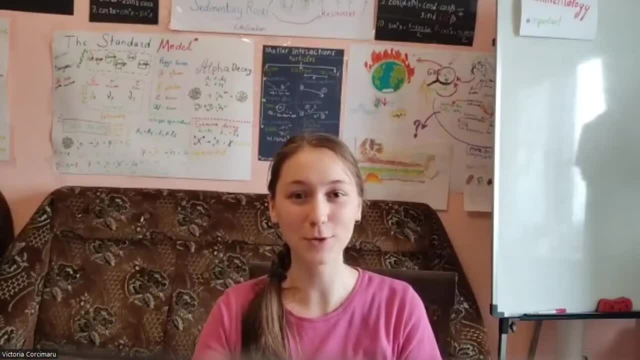 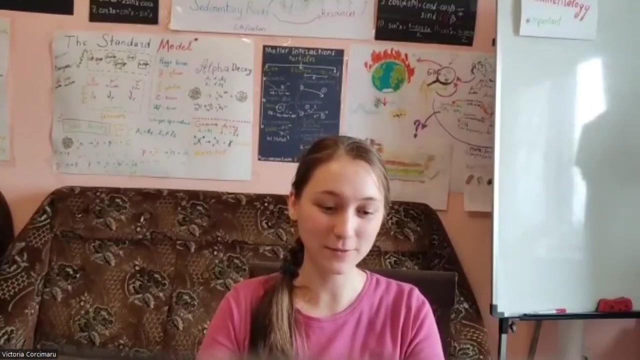 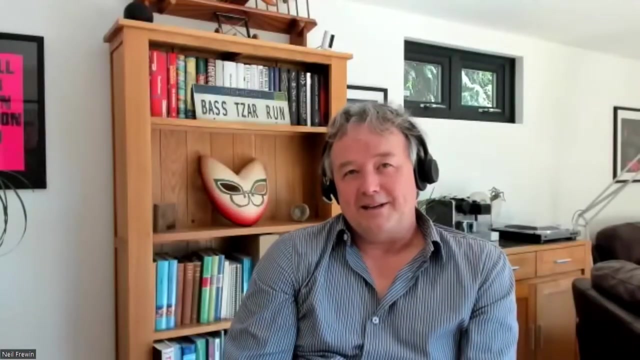 attractive to people my age who are so into computer science and it and technology. so i was wondering if you could give an example of something tangible or something from what you have seen or done that could. that could give a sort of feel for what it could be. yeah, i can do. it's um. i mean data science, of course, is a whole. 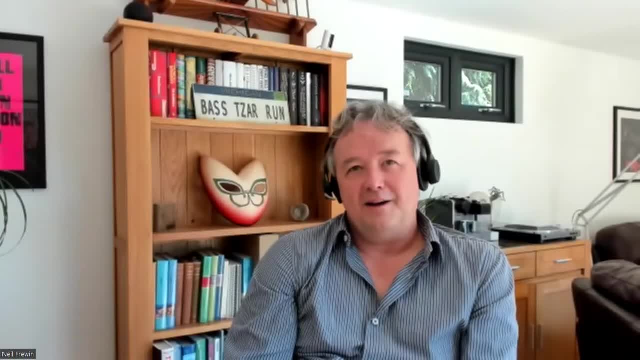 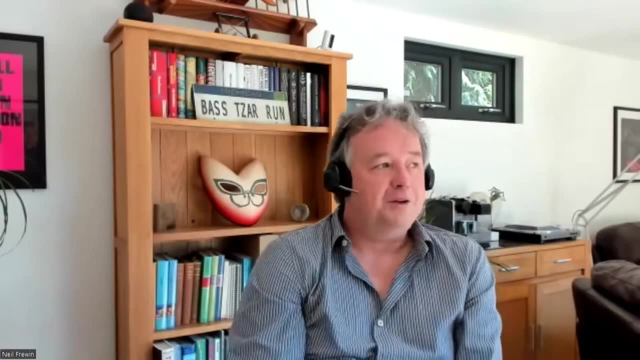 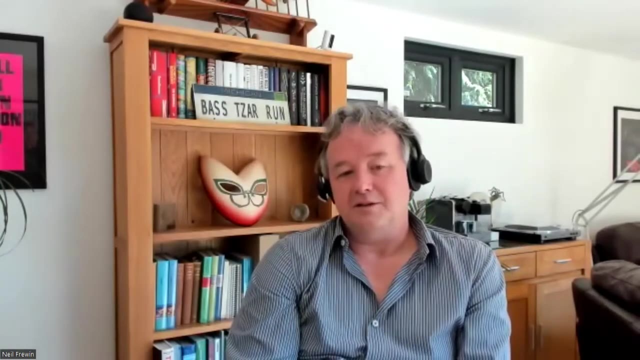 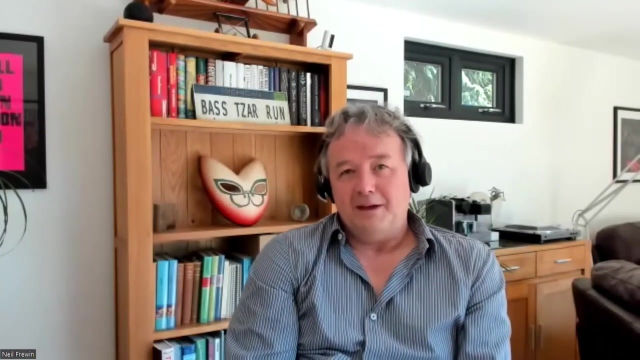 new arena and i think many, uh, you know, people coming through universities these days and into the workplace are more and more being expected to have a background in, you know, python, coding, um, or some appreciation of computer science and and how to manage large bodies of data proactively. And so we see it more and more, I think, in our world, in my world. 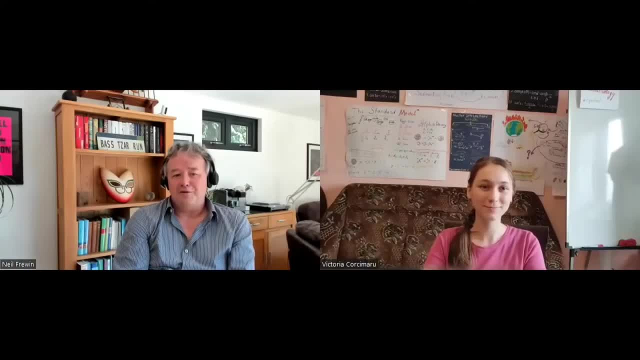 I mean I'm not very good at savvy. I must say I've been through a Python course And apart from knowing what Python means, at the end of it I probably couldn't do much in the way of coding. But certainly those that are in that world can really do some nice. 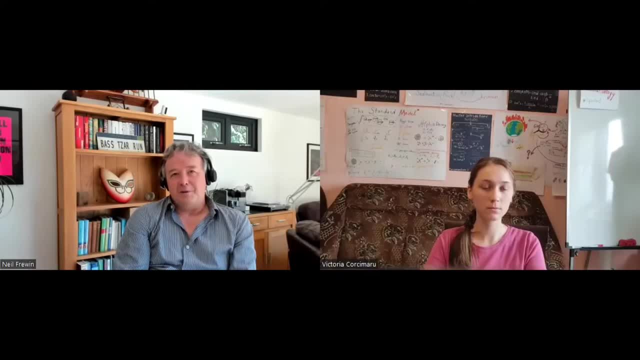 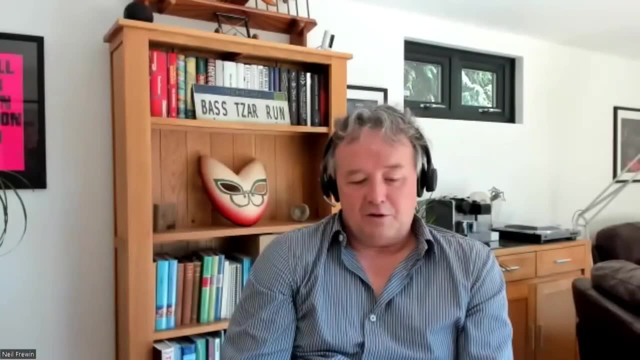 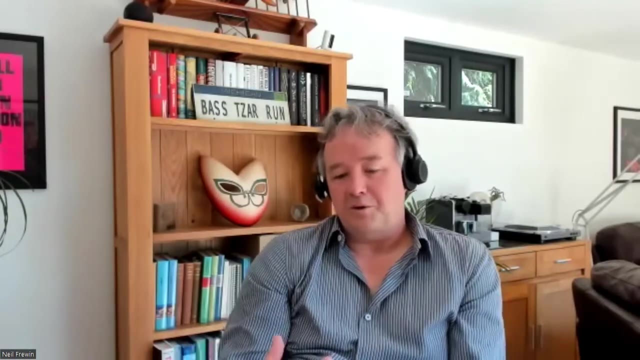 things And it's kind of and a lot of problems are being solved on the fly. at the moment. There's a large community in this company of machine learning and artificial intelligence enthusiasts who are really thinking about how you can learn from data and how you can 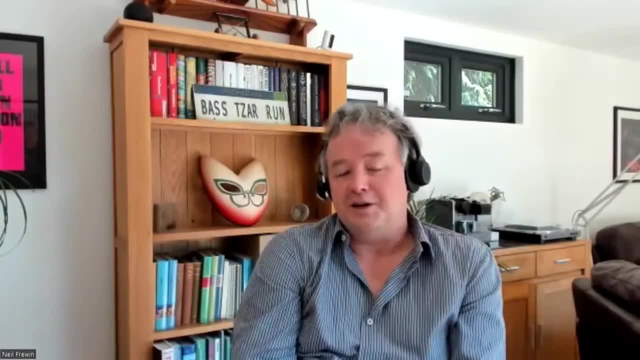 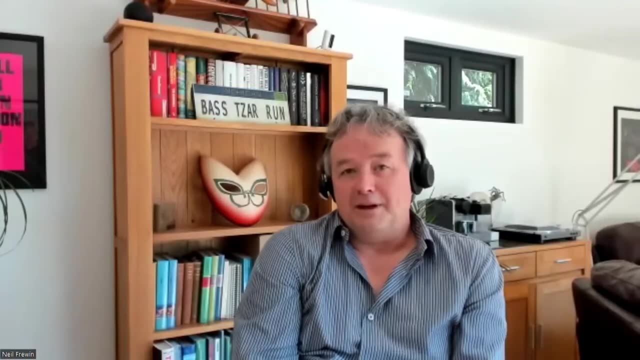 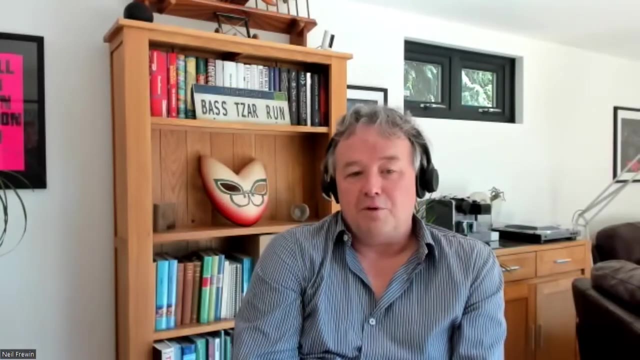 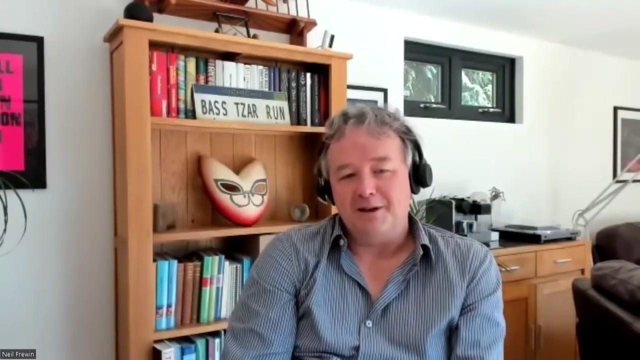 even potentially get to drilling- a prospect- just using machine learning and artificial intelligence. So, for example, there's seismic interpretation associated software now that, uh, that will learn from prior interpretations and uh and and draw your interpretations, new interpretations for you on the on the seismic, having learned a little bit about. 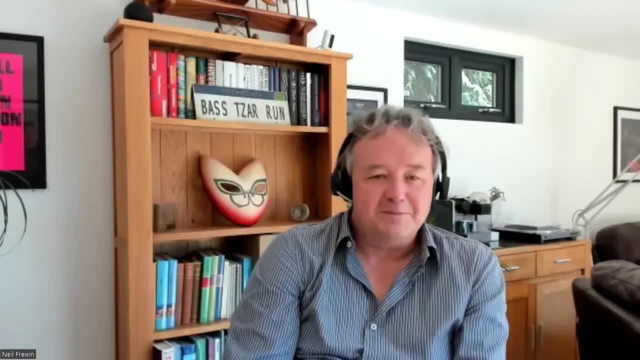 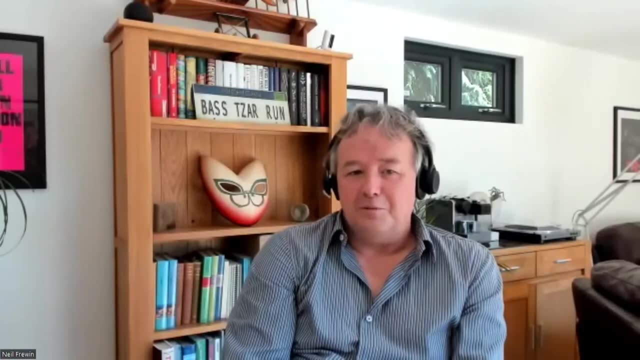 what you've already- uh, you've already- identified as features on previous seismic interpretations. so, um, so, none of this takes the human out of it. the human component is still very important. we're still dealing with nature, after all, and nature is not always the most predictable. um, so you do. 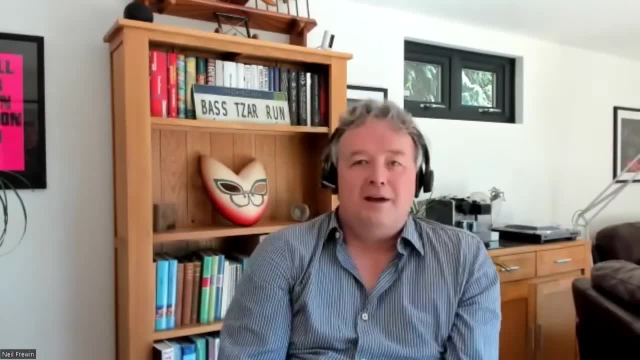 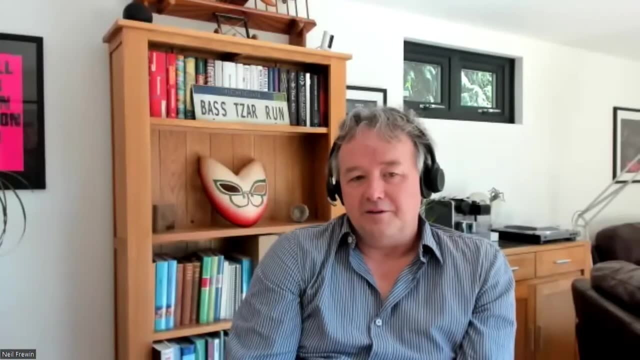 still need to have the human element in there, i think, but more and more i think we're able to use the data that we have access to, to uh, to to build a, a truly digital earth and uh, and i think that's that's really coming together very well uh at the moment and will require, i think, still a lot of. 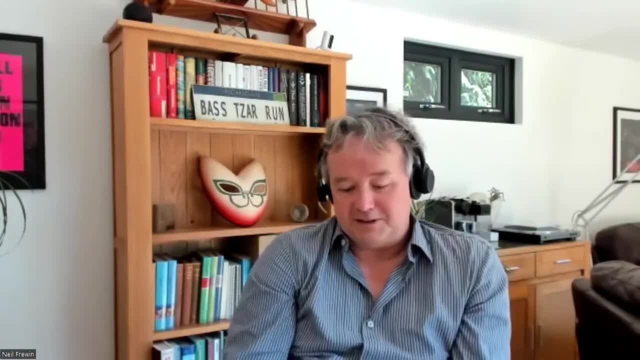 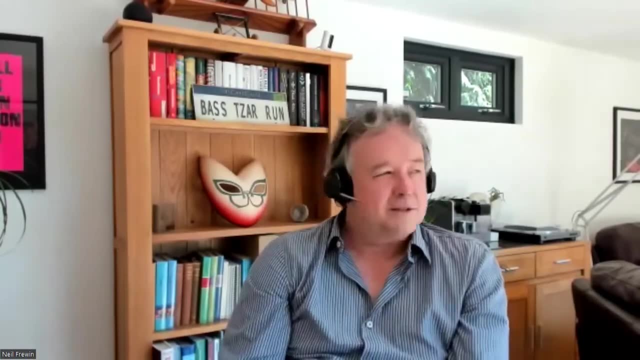 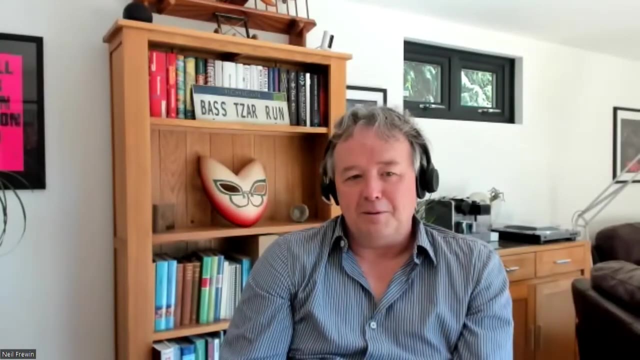 work to do that. so i'm hoping there's still, you know, continued investments, um, in geoscience to allow us to see that that story through and really bring the data together. i would say that, uh, the geoscience data is probably some of the more difficult data, uh, that you can really play with, i mean, if you work. 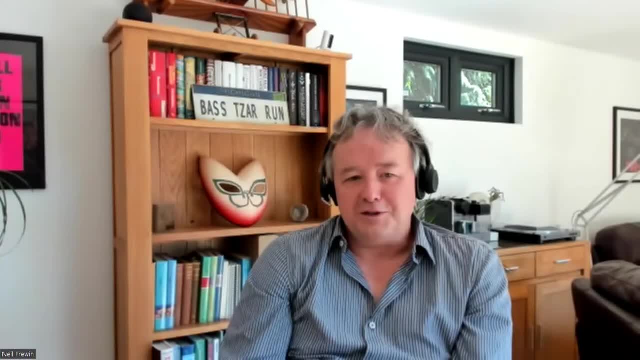 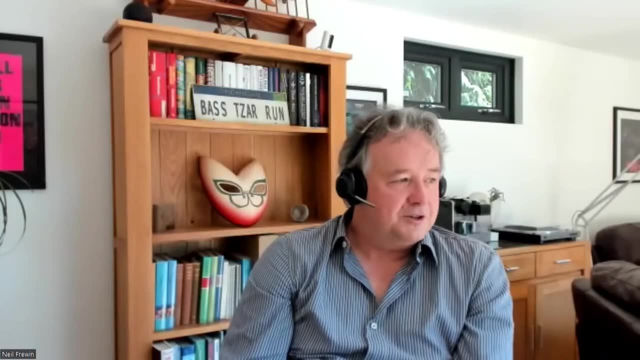 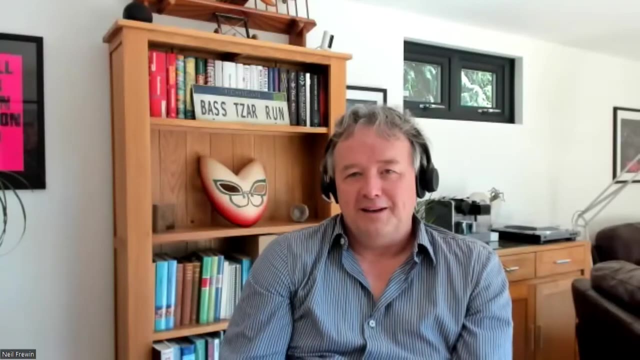 for amazon. um, i think the data trends you see there are are are data you can harness and control in and, of course, in in in geological and geoscience data. it's very hard to uh to really integrate that fully because it depends so much on on so many different factors that you've got. 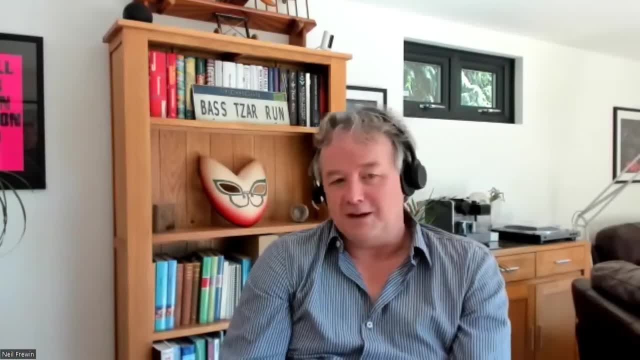 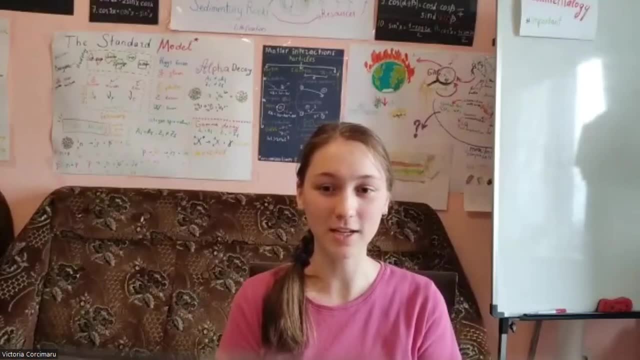 to consider and bring together um, so, so fixing that is really it's really important and the data is really important and the data is really important and the data is really important and this type of data analysis is exactly what you need when it's getting harder to access those. 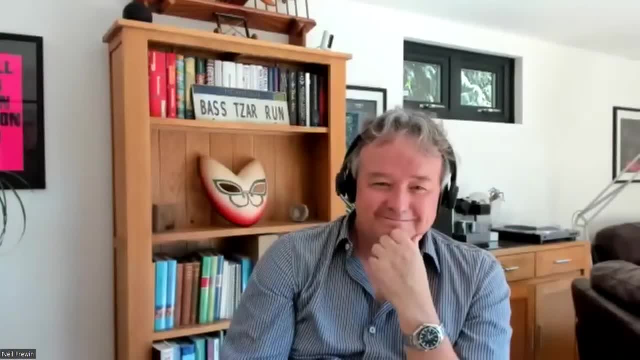 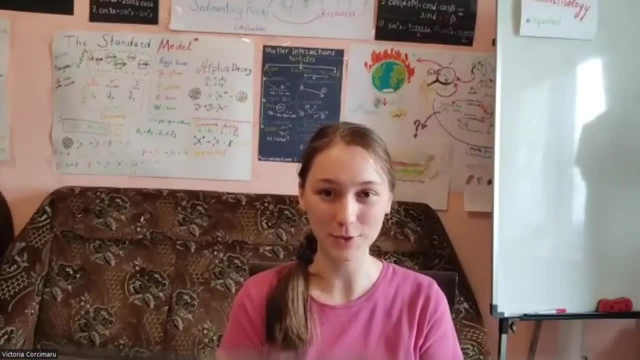 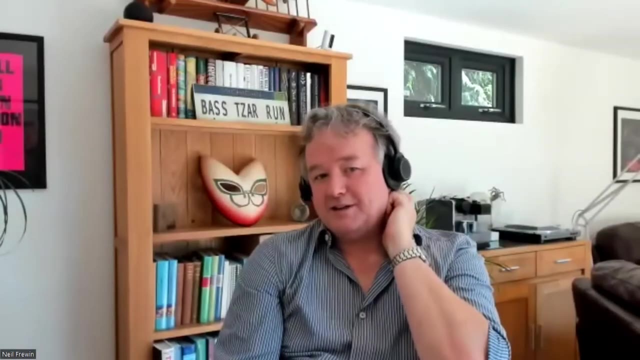 hydrocarbons and yeah, when you need to make sure your project is actually going to be profitable and safe and all of those other check items on the list. yes, yeah, you need to. it's it's more and more about integrating that data and bringing it together and uh, 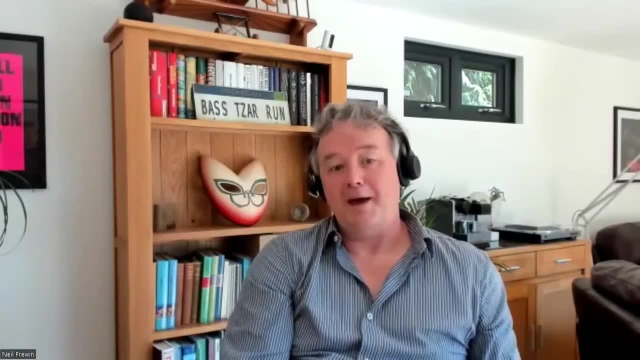 and almost. uh, you know, avoiding the pain of the data, and the data is going to be more and more uh and more about integrating that data and bringing it together and all of those other check items on the list. yes, yeah, you need to having to do that. uh, having that ready in place for you to really do the new thinking around what's. 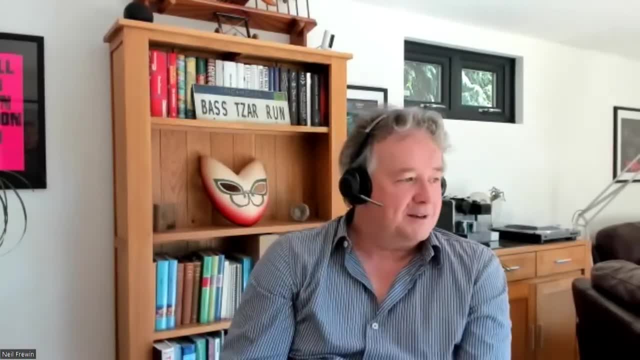 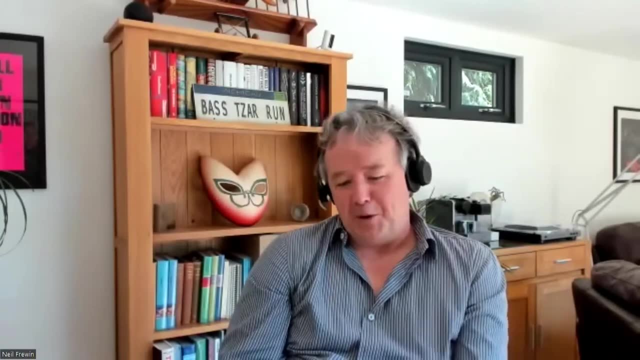 beyond that existing data set. uh, we have that phrase in in this company. moving beyond commodity knowledge. um, so, commodity knowledge is something everybody has. you're moving beyond that into something that's that's your knowledge and uh, and you've created it out of uh, out of the gaps. 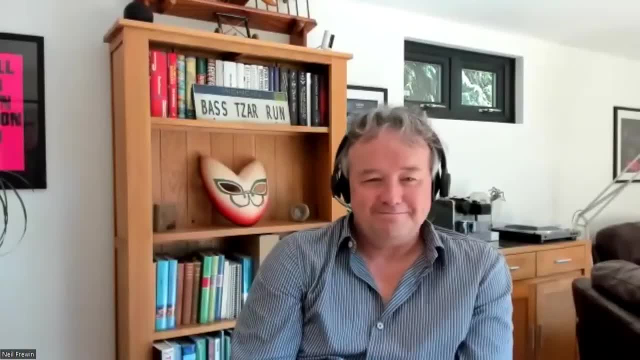 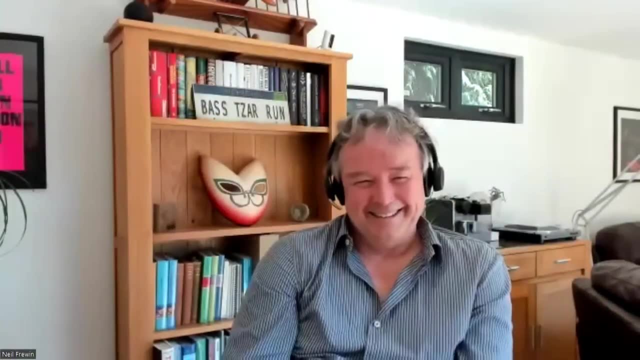 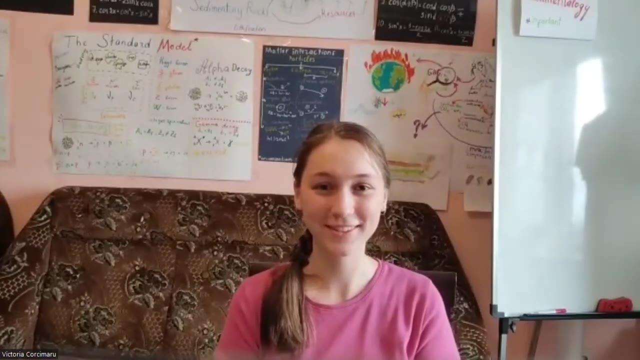 uh that you've seen in that data set. wow, that that is a very smart thing to say. smart, not the for a company. yeah, i can see why she was so successful is it? is it fun to work for shell, do you? do you like your job? i love my job. i've always loved my job. it's uh, it's uh. it's been a great. 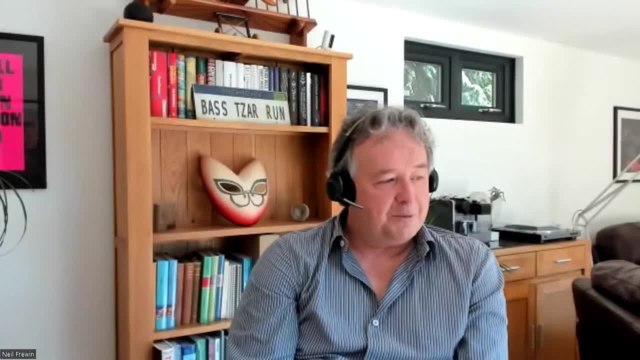 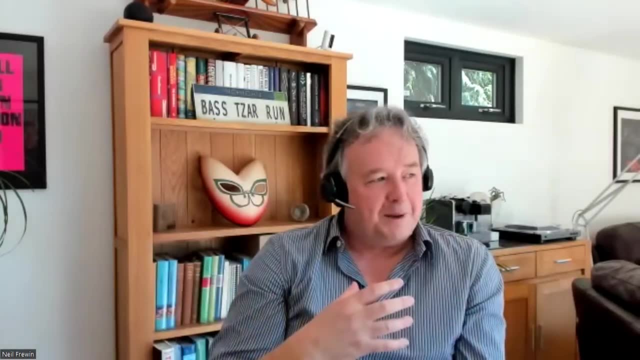 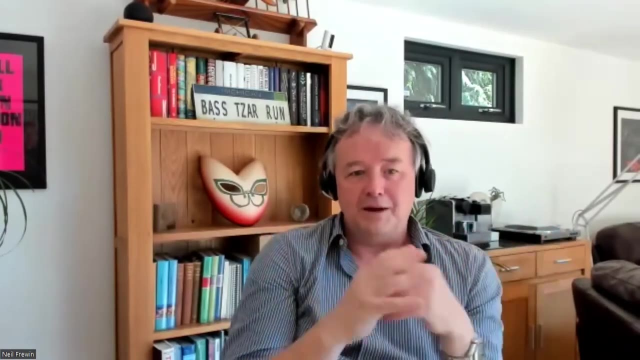 company to work with. um, you know, it's interesting when you uh, when you hear uh, because we're subject to so much perception. um, you know, social pressure these days is quite strong and uh, and with a brand like shell, you know which is a you know billion, multi-billion dollar brand, uh, it's sometimes a very easy target, but, uh, i've yet to. 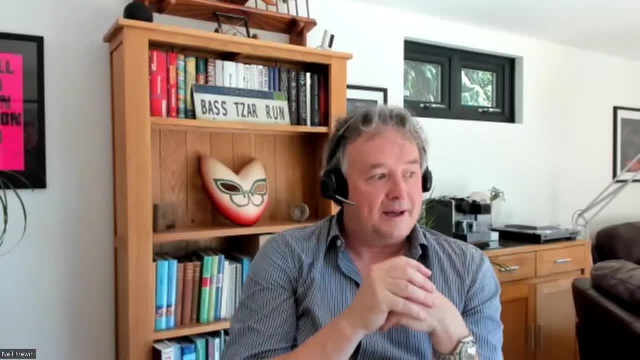 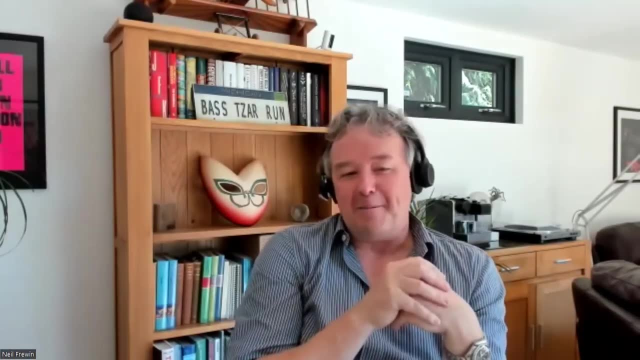 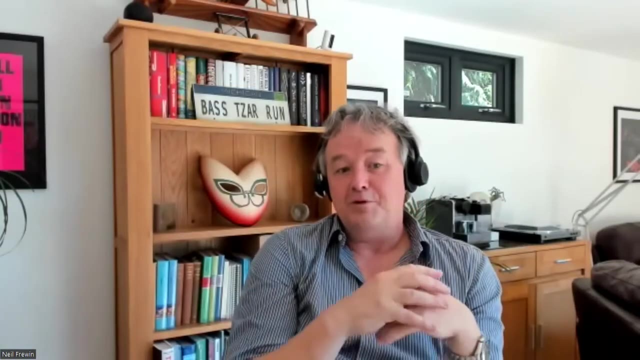 meet anybody in a company like shell uh, or as shell that, uh, that that uh, have any, any other, any other intention than good intention? um, in a company like this, and so, uh, and in fact i, you know, i often think that geoscientists, people like us are, i have the most understanding of the planet. 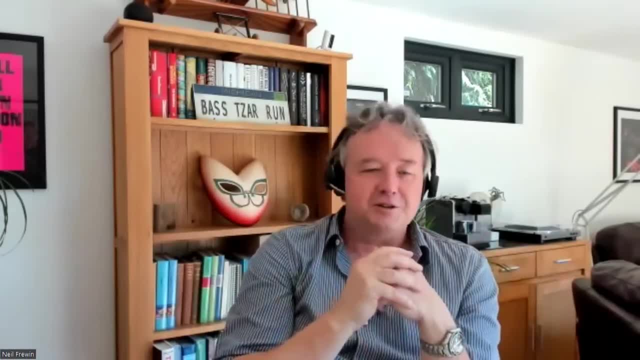 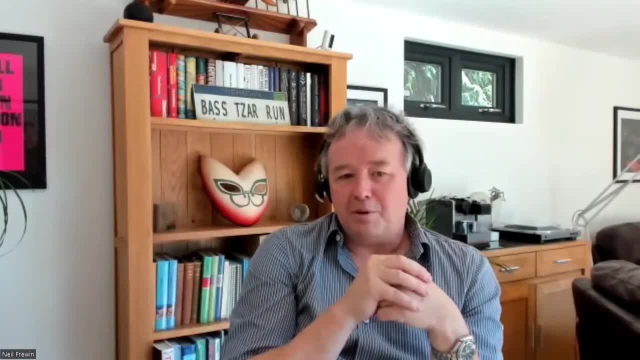 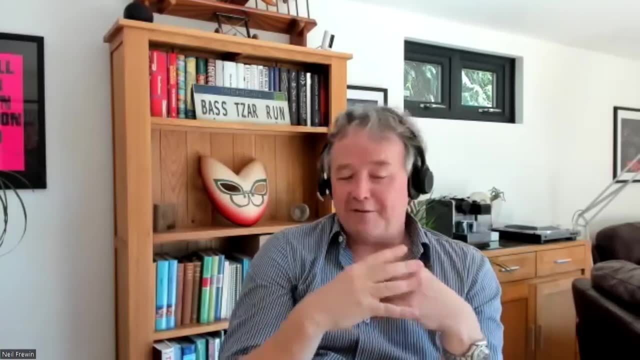 of years and so, uh, so most of the people i work with probably have the greatest appreciation for the planet in which they live than anybody i've met anywhere else, so it's it's so that for me makes a very nice place to work and, uh, because they share my enthusiasm and interest in in the 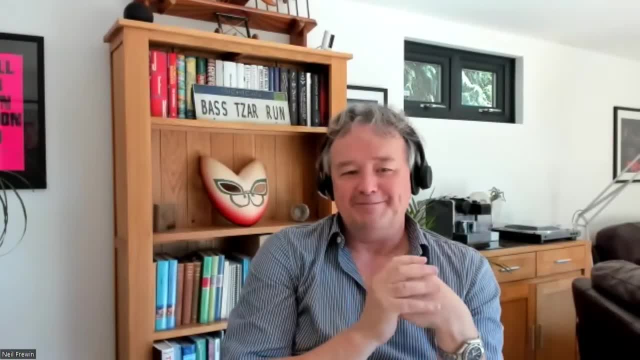 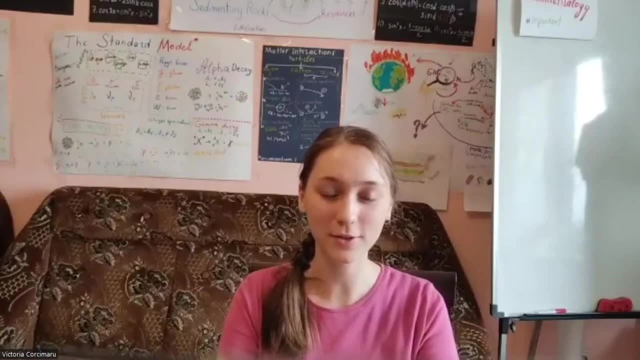 earth. so it's uh, yeah, that is. that's truly great. i do enjoy that. that's wonderful. as i've been listening to your answer answer, another question came up. you mentioned that you have such an appreciation for our planet and granted also a lot of knowledge regarding it. would you say there's a lot that we don't yet know about our planet? or, like percent? 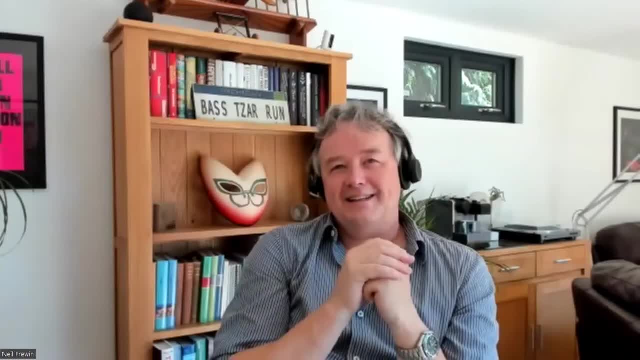 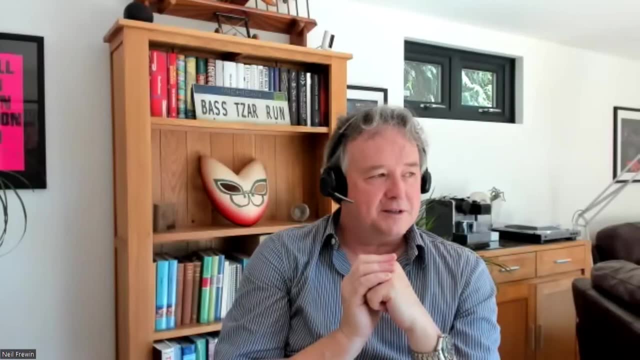 wise. how much? yeah, yeah, that's, that's an interesting question, because, uh, i did, uh, i was writing an article, uh, a few years ago and i i coined the phrase, uh, peak geoscience, because, um, and this was really a bit of a ploy to get people to put abstracts in. 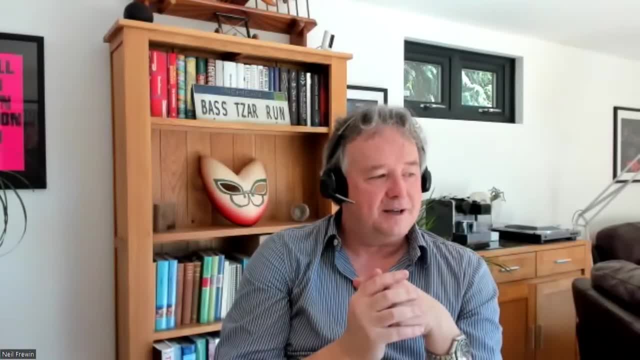 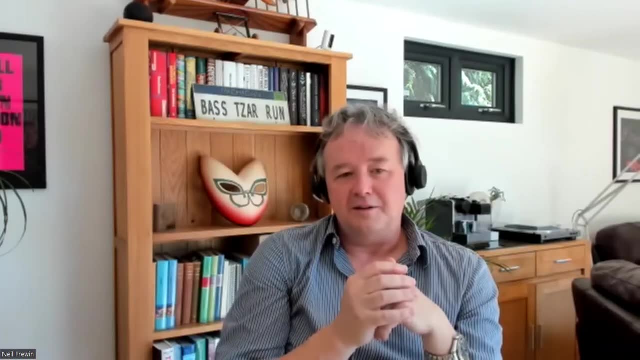 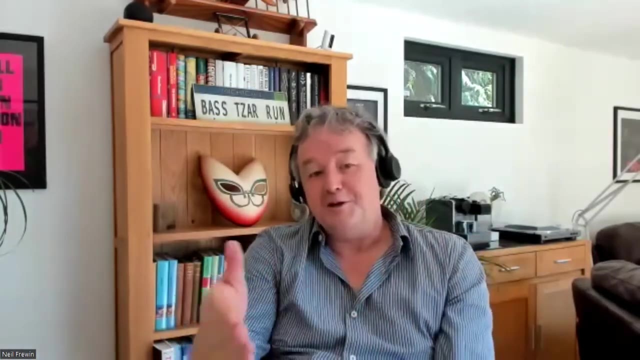 for a conference. but uh, so i i challenged the community to think of, uh, any really fundamental recent advancements in uh in geoscience, that, uh, that would really alter our understanding of the planet. and, um, you know, i spent some time trying to map, you know, the changes that we've seen uh. 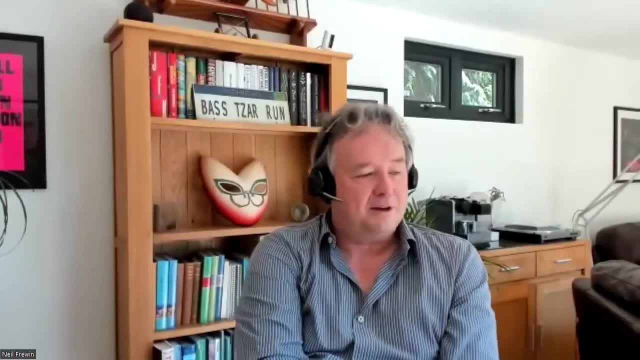 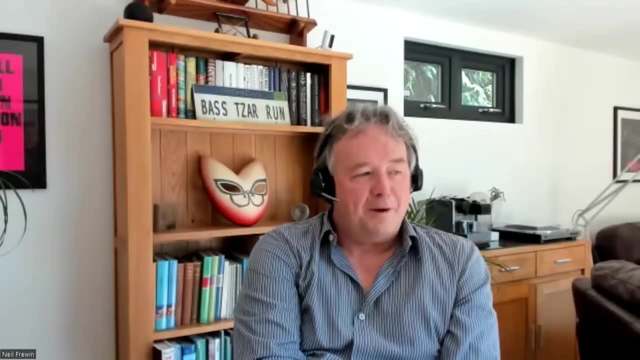 let's say, the fundamental changes in our understanding of the earth over time, and i would argue they're getting fewer and fewer actually. so, uh, um, now that i'm always, i'm always hopeful- people disagree with me on that point and uh that they will say: wow, yeah, but 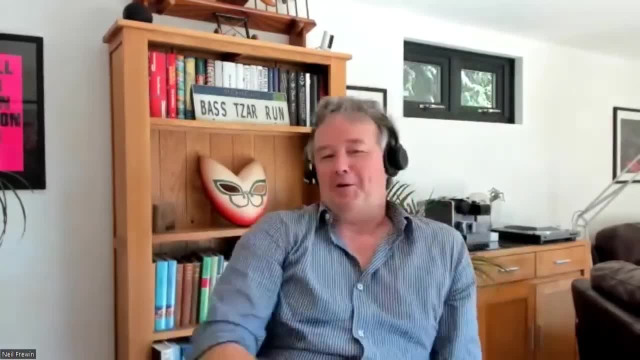 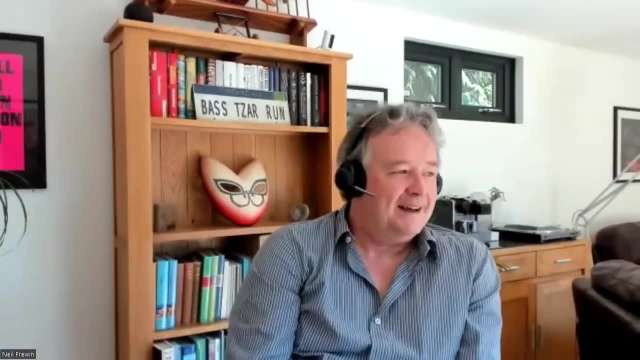 you've forgotten about, uh, this topic that, uh, that we've been working on now for the last 10 years, and we're about to publish this amazing paper and, uh, it's going to completely change the way you view the earth. um, and i, and i hope that's, i hope that's the case, but, um, but i've, i've, i've not seen. 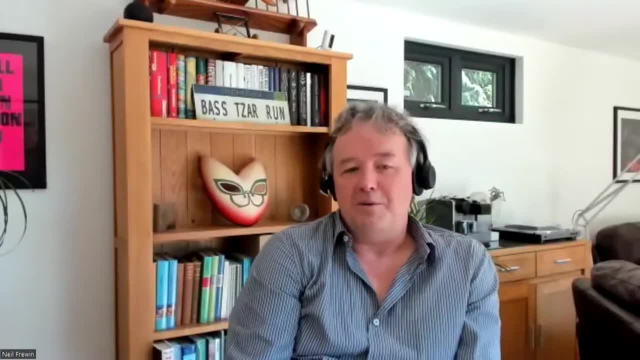 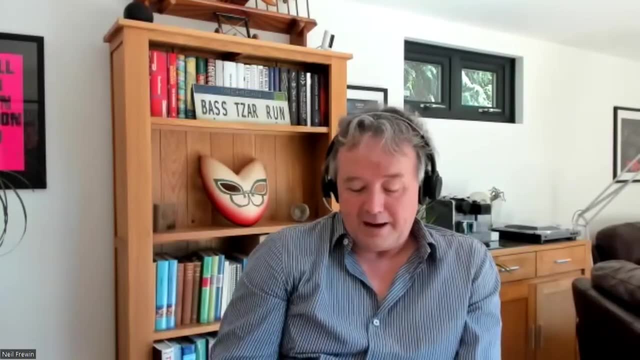 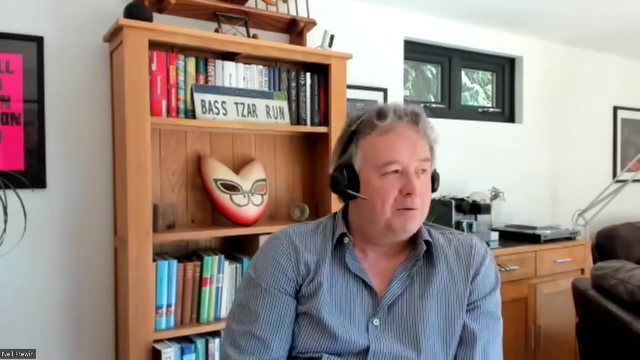 anything uh too fundamental coming through in terms of the way we we change that view. i think the most fundamental changes in our, in our science, will be seen now the way that we see anthropogenic climate change, um, now, our impacts on the planet, i think will be probably some of the more fundamental changes in in understanding of science. uh, that. 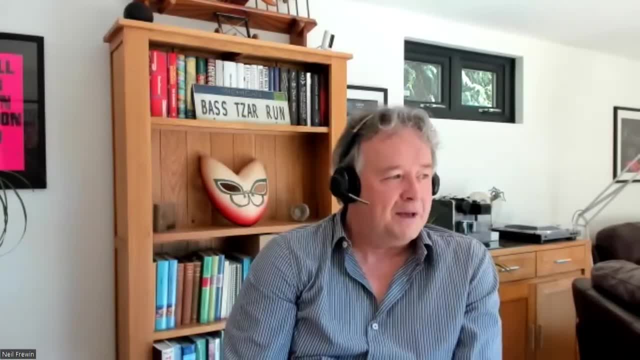 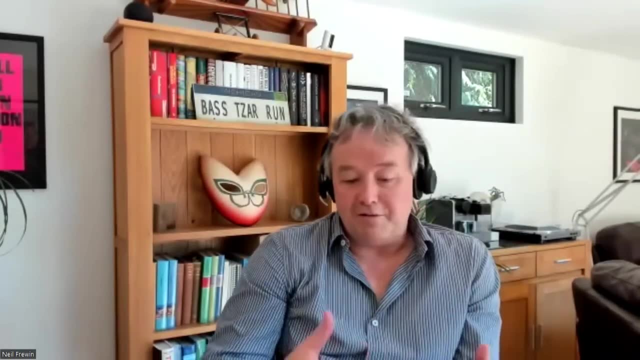 will still come. i think, uh, you know we see a lot of, uh, there's a lot of strong evidence now, i think, for anthropogenic climate change. there has been for some time and that body of evidence has been growing and growing and, uh, i think, the more we can do with that and understand our own impact on the 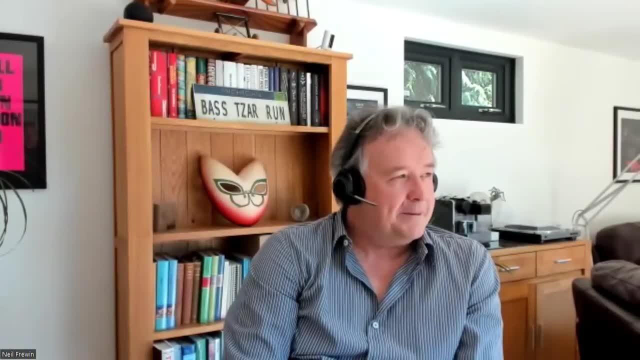 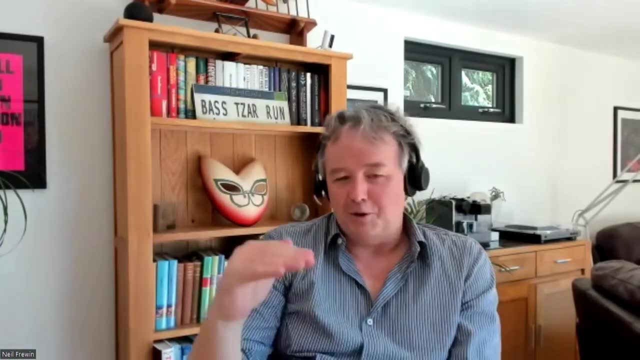 planet, the more significant it will be. there was a paper by um as an article i saw recently by professor phil ringrose, uh, that suggested, uh, you know, changing the way we look at the geological time scale and really enhancing the most recent, uh, you know, a few hundred thousand years, and trying.